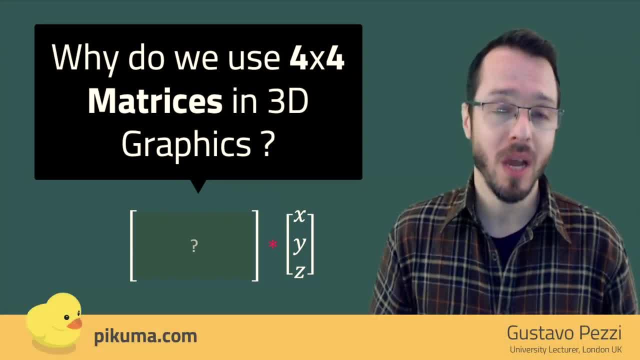 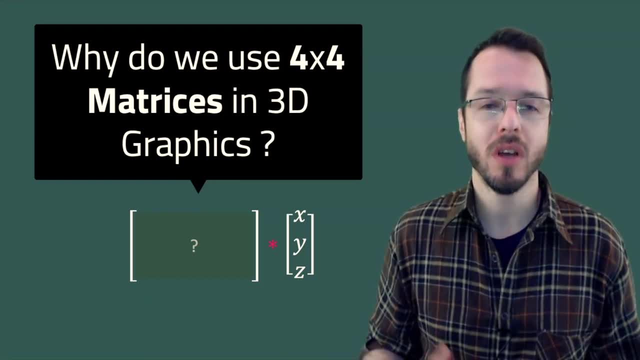 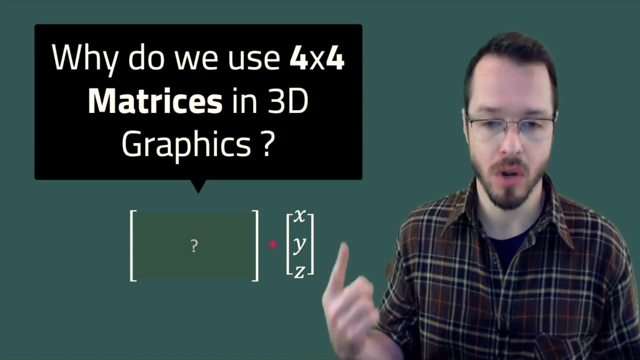 Hello everyone, Gustavo here. So today I want to discuss one very common question. whenever we are programming 3D graphics, Why do we use 4x4 matrices? whenever we want to apply transformations in our vectors? So we have our points, our x, y and z points in space Whenever we want to. 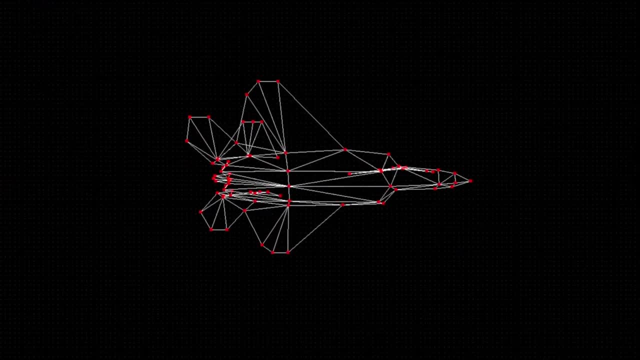 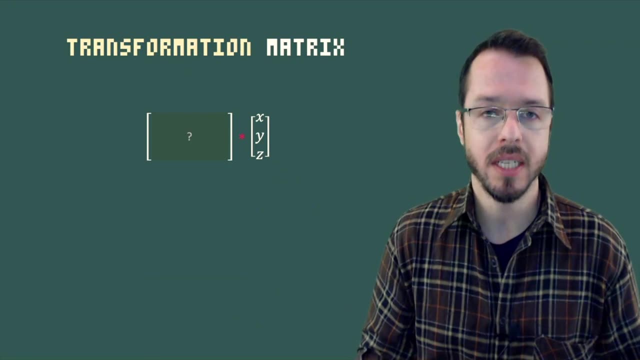 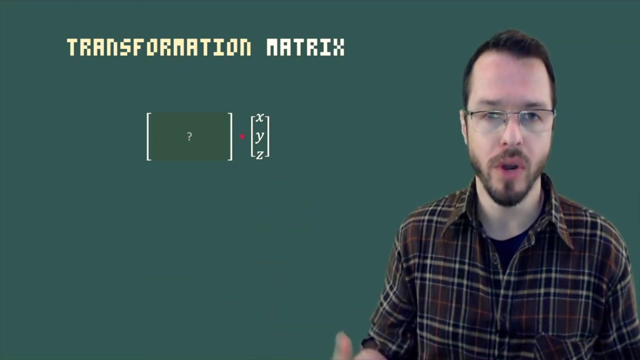 apply transformation. rotate scale translate. why are these transformations encoded in a 4x4 matrix? We use in computer graphics these ideas of matrices, right? So in our course we have been seeing that we use a matrix. we multiply that matrix by our original points, our original. 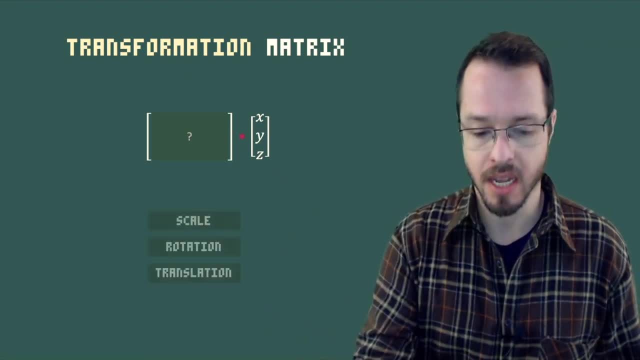 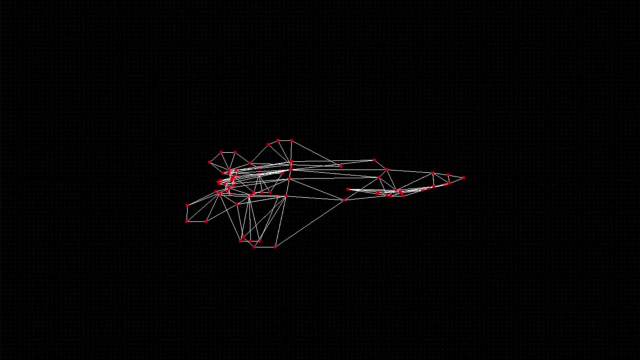 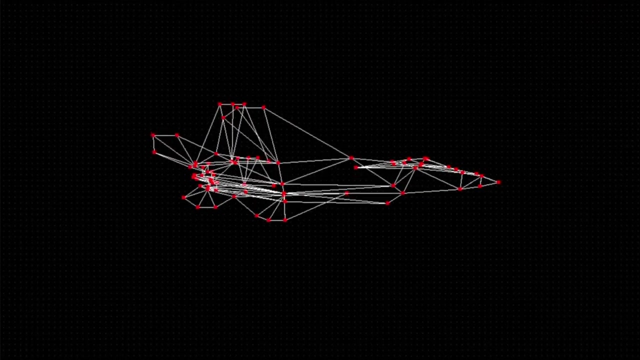 vectors and then this multiplication. right here we have things like we can scale those vectors, we can rotate things, we can translate them around and all these transformations on our original points, they happen by multiplying a matrix, right? So we have this matrix. 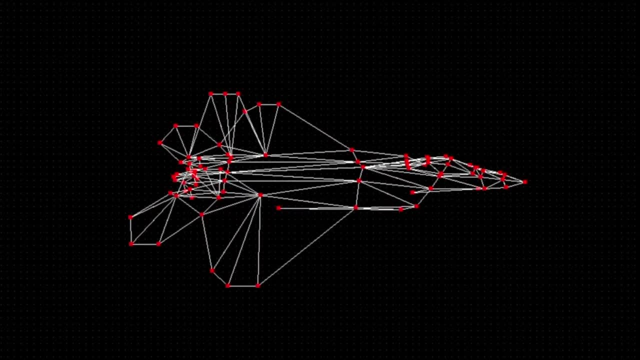 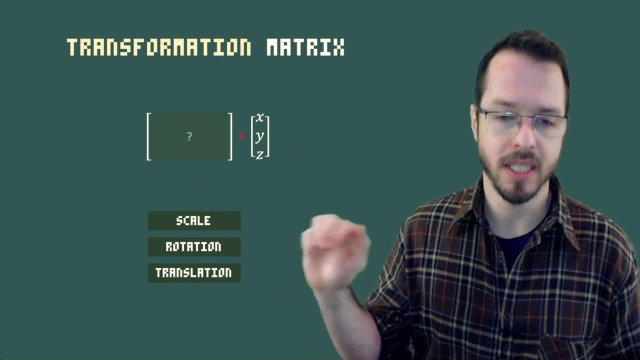 that we go, we multiply by each one of our little dots and we know that, depending on the values that we populate on this little matrix right here, whenever we multiply, we are going to perform a scale rotation or a translation in our original vector. All good, so far Right. but the thing is: 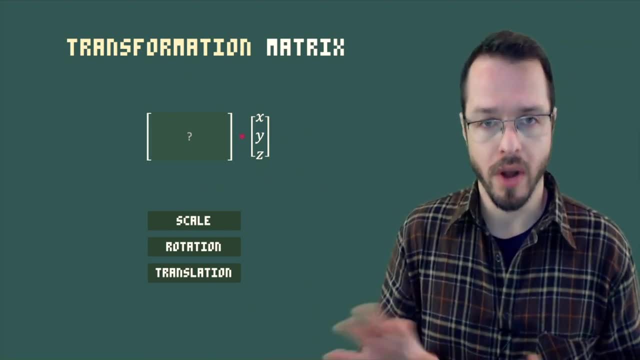 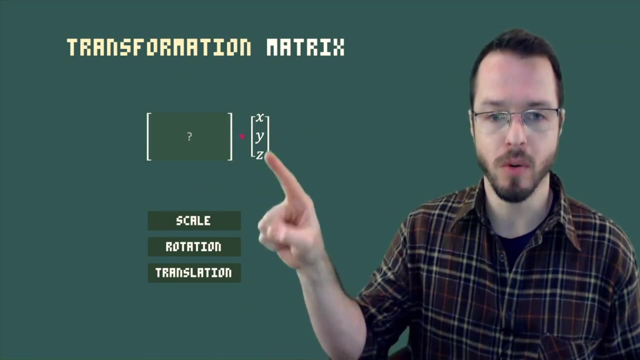 I told you also, and we also saw whenever we were coding our 3D renderer, that this matrix right here, we use a 4x4 matrix and not a 3x3 matrix whenever we're multiplying by this original vector right here. And the reason why I took the liberty of recording this video is because I want. 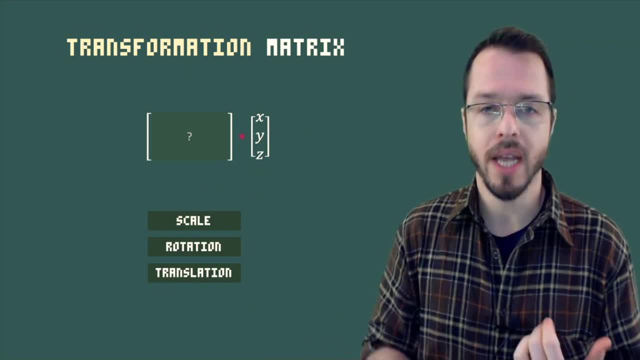 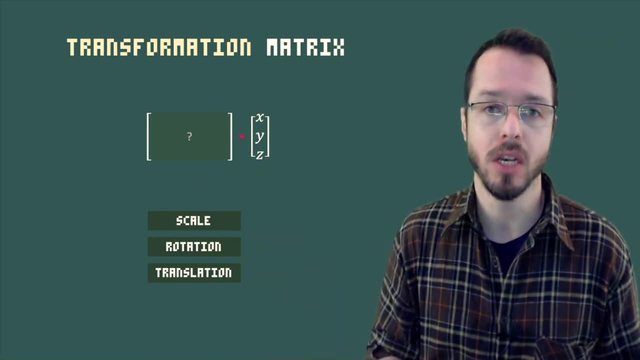 to talk to you about the mathematical reason why we have to do that, but also I want to give you some intuition, right? So I want you to visualize why do we have to use a 4x4 matrix and not a 3x3 matrix? And I'm going to give you a spoiler: If we were talking about these three important 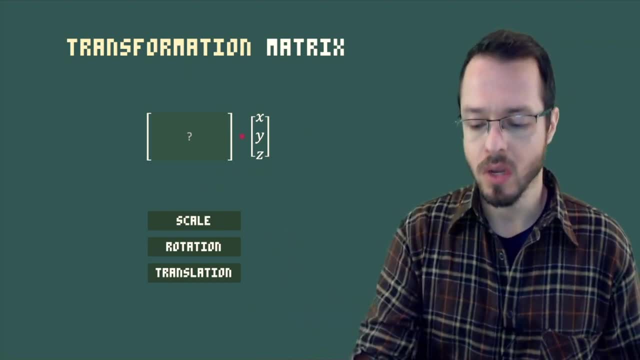 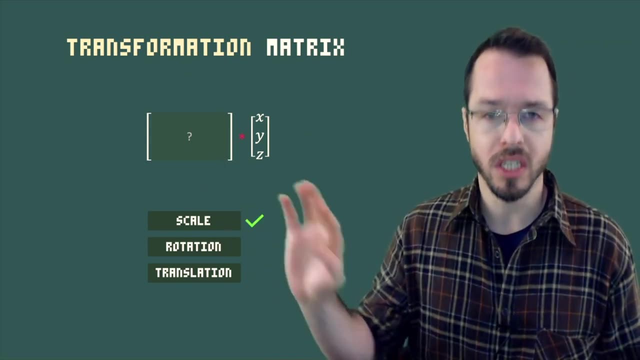 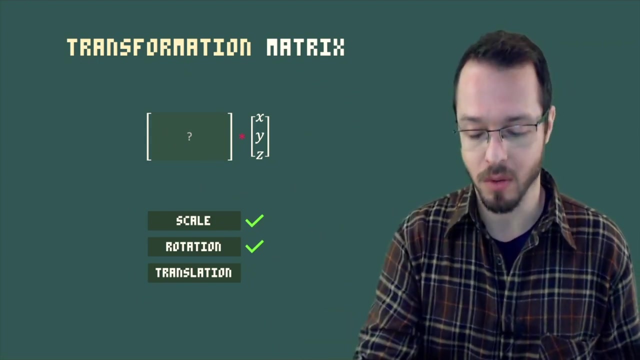 transformations, scale, rotation and translation scale. we could use a 3x3 matrix. that will be okay. the only issue here is translation right. Translation is the weird one out, So translation. we cannot simply use a 3x3 matrix to represent translation right. So this is the one that I'm 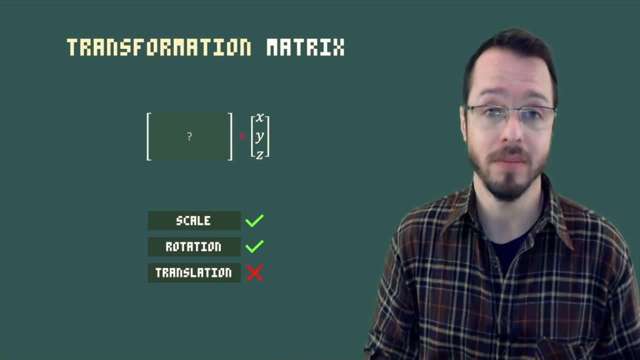 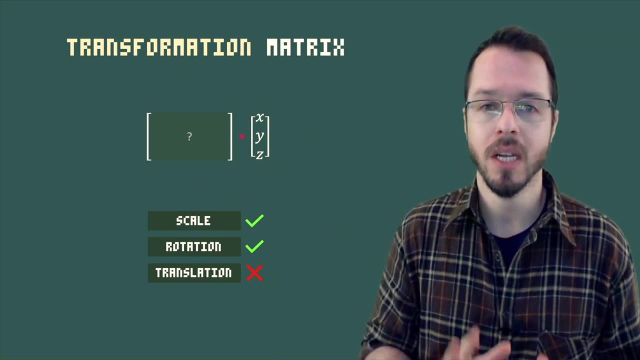 going to zoom in and try to explain why translation is a little bit weird, right? It's different than the others. So what I want to do right now is I want to pause and I want to zoom in into translation. Let's just look mathematically: What does it mean for us to use a 3x3 matrix? Well, I'm going to. 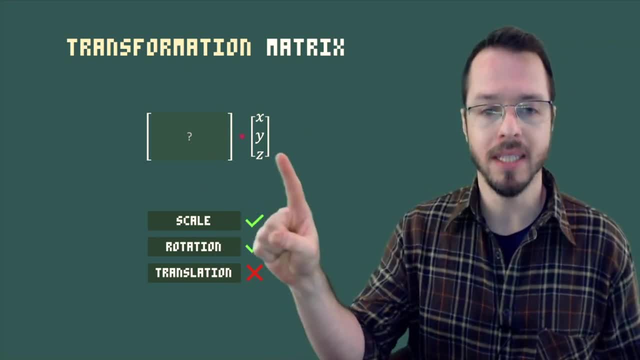 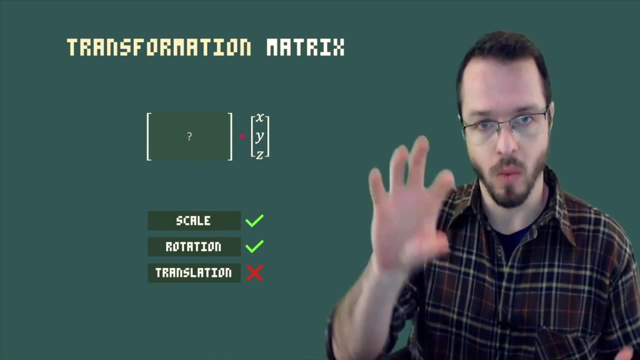 explain why translation is a little bit weird, right? So we multiply these things and translate x, y and z, right, Our original vector: x, y and z translate by an amount in x, translate in y and translate in z. So let's look at translation. 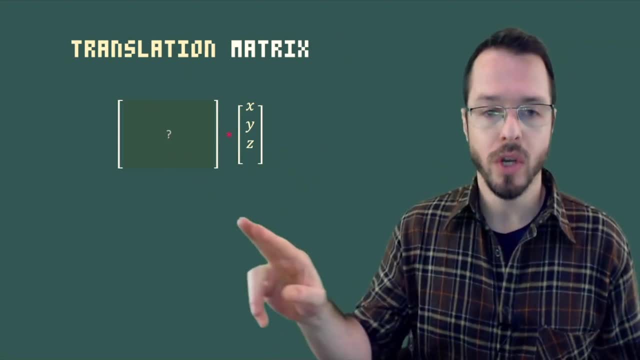 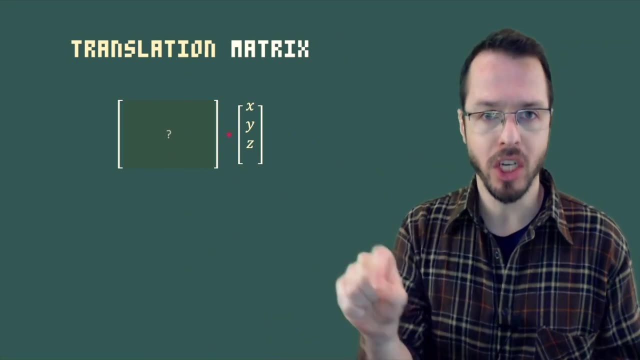 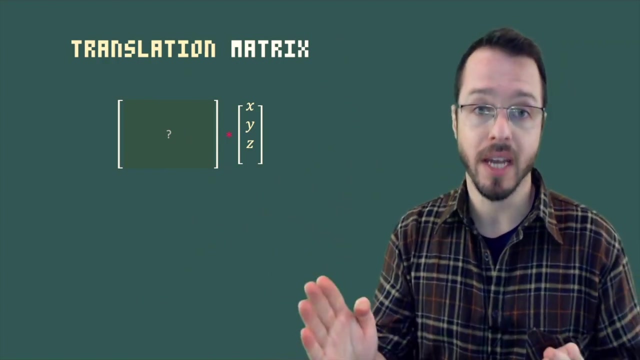 matrix. We know that our goal is. we want to find a little matrix that if we multiply by our original point x, y and z, right, We have all these points of our mesh. And then if we multiply this matrix by every point, we want to translate all those points. We want to translate those. 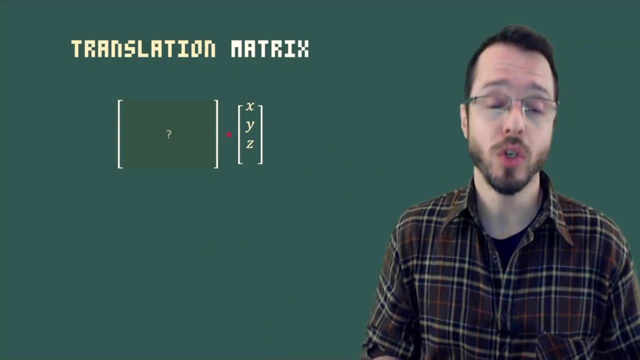 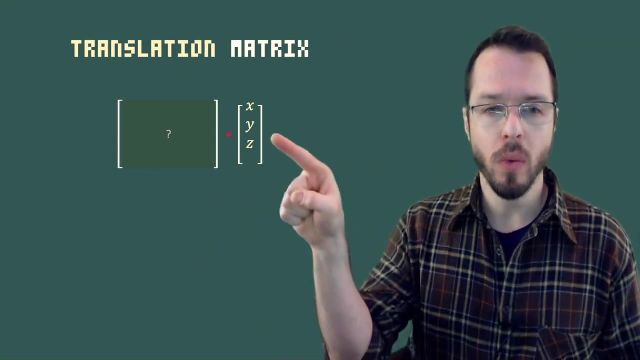 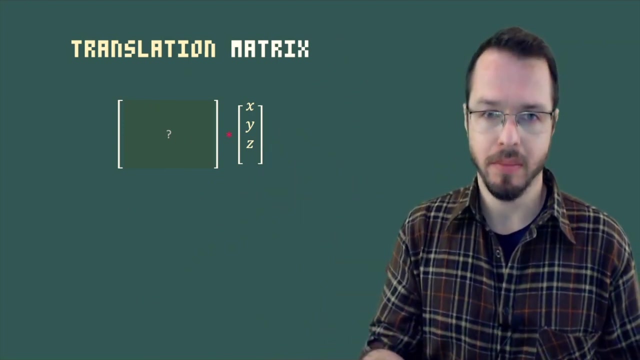 vectors in our 3D scene And I told you before that for us to be able to translate. do you agree that for us to translate something- x, y and z? we want to basically add something to x, add something to y and add something to z. That is what translation means. right, I want to get those. 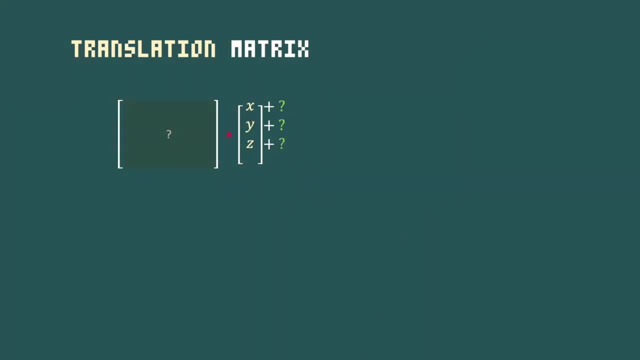 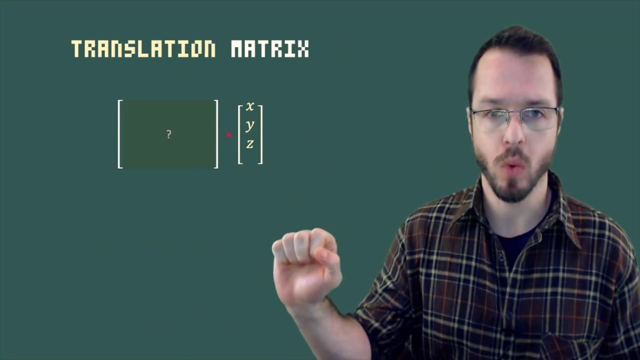 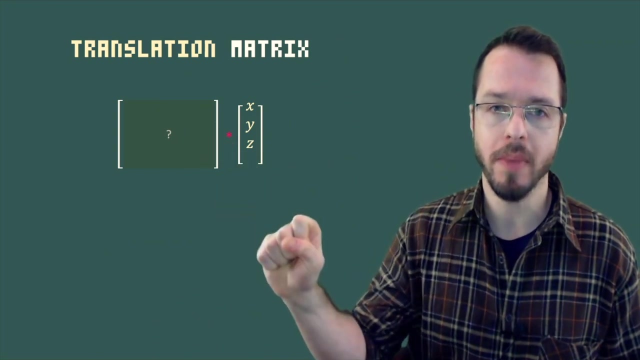 values and I want to offset by a certain amount. So I want to add something to x, add something to y and add something to z, And if we stop and we look at how matrix multiplication works, we cannot achieve this. x plus something, y plus something and z plus something only with a 3, by 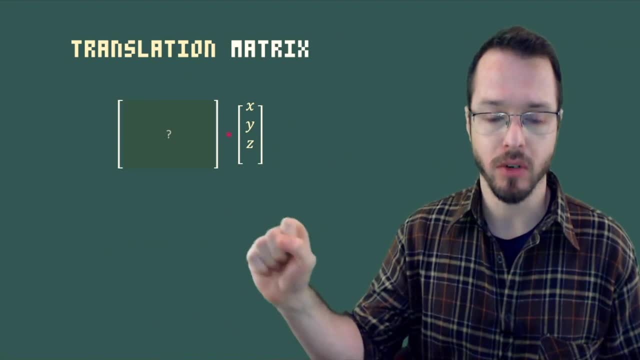 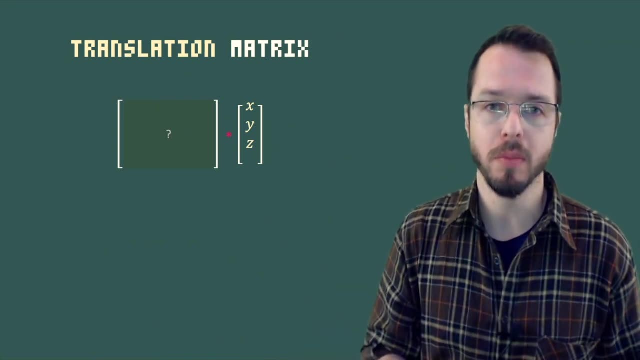 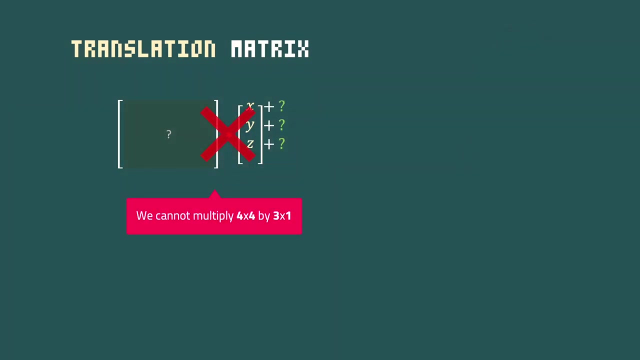 3 matrix. We need an extra set of components to this matrix, So we are going to have to use a 4 by 4 matrix. okay, And also we know that one of the rules of matrix multiplication is we cannot multiply a 4 by 4 matrix by a 3 by 1 matrix. So we are going to have to add an extra little component. 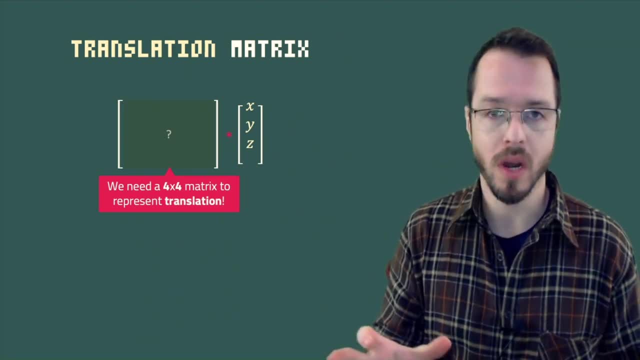 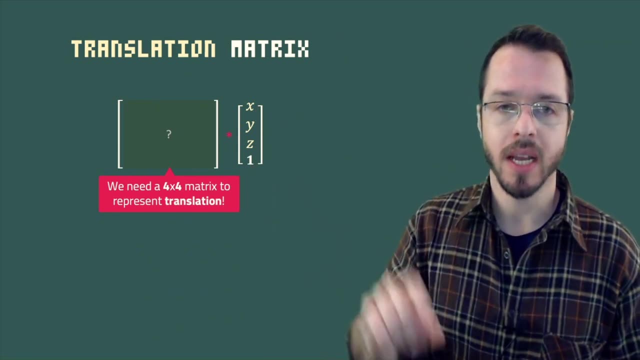 for our matrix to represent translation, right Translation is the odd one out And I am going to have to expand And instead of having the original values x, y and z now I have to have one more extra component and it's going to be x, y, z and a little. I'm going to put a little neutral one. 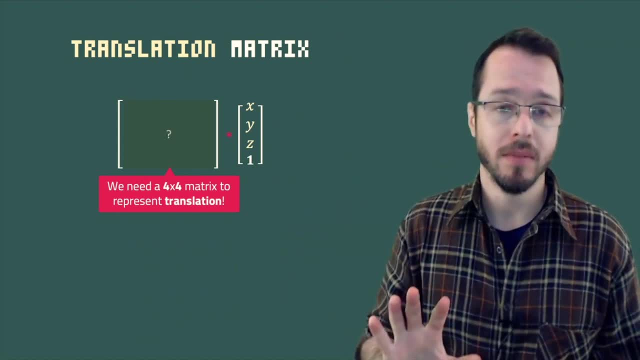 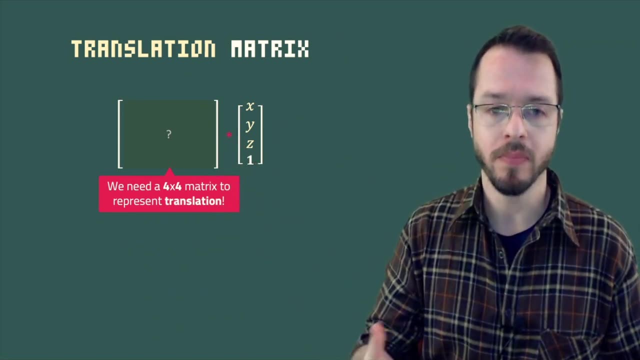 there to be our little fourth row Right. So now that we have this 4 by 4 matrix and we have this extra little component for us to be able to multiply this matrix, we need to understand, understand that the whole. if we open this multiplication between these little black. 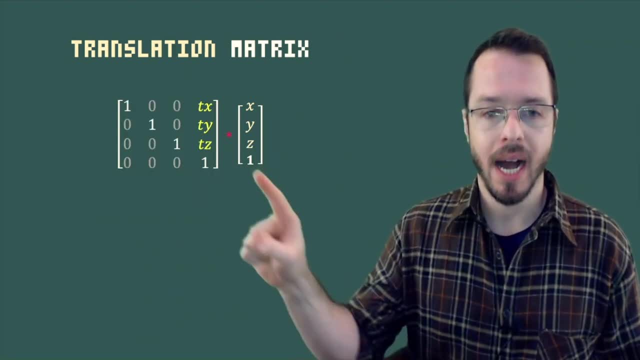 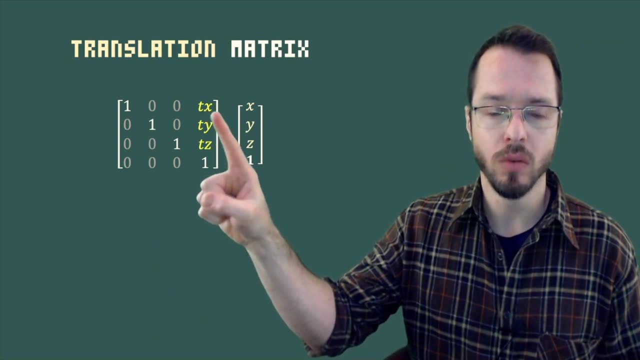 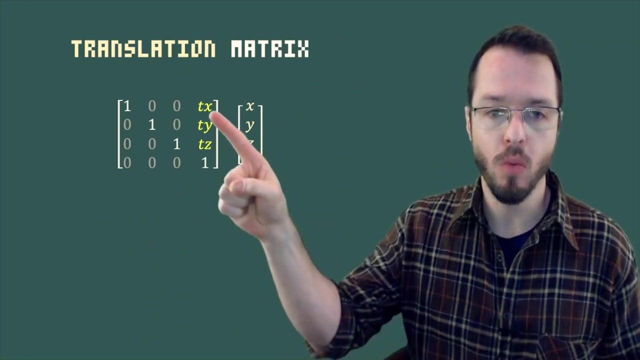 box and our vector. this is what we get. I can populate on this last column right here, on these values, I can add a little: translate x, translate y and translate z values, right? So these are going to be numbers that I can say how much I want to translate in x, how much I 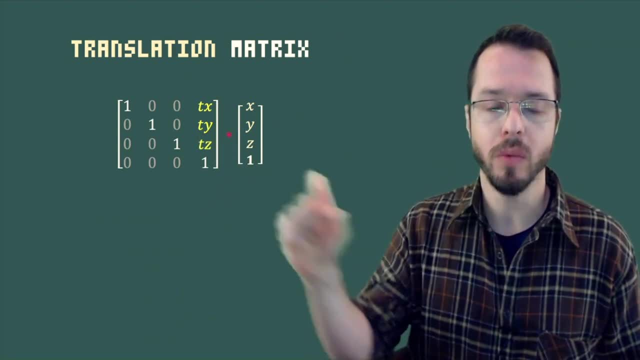 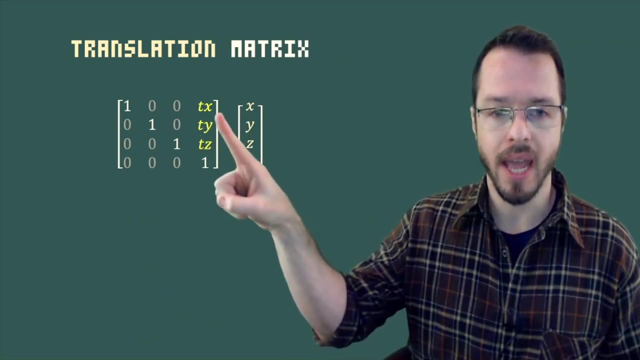 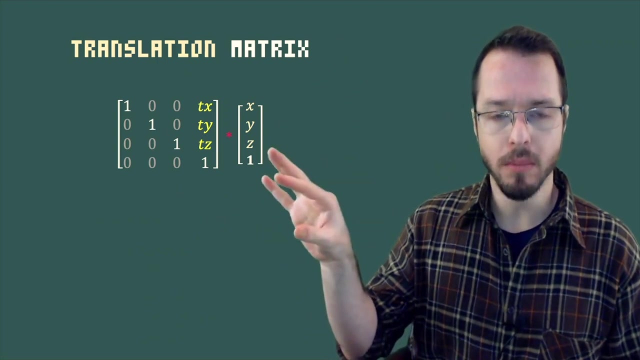 want to add in x, how much I want to add in y and how much I want to add in z. So if this thing right here, if I keep the identity matrix with ones in the diagonal and I add on these last column here the little amount that I want to add to x, y and z, if I open the 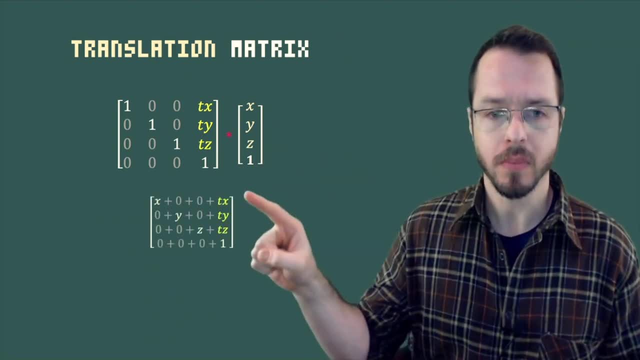 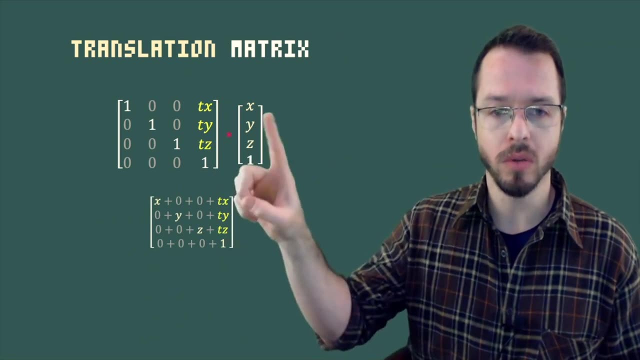 multiplication. it's very clear why this works, because remember that matrix multiplication is. I get the row times the column and then the row times the column, the row times the column. right I have the little multiplication between rows and columns, and I already expanded here. 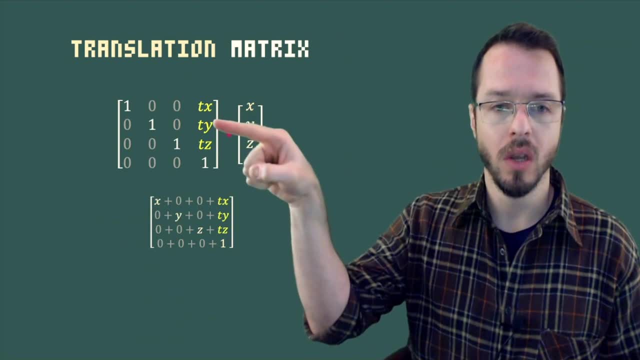 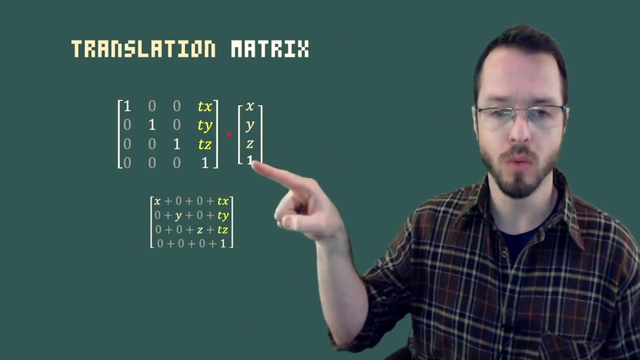 and you can see that this is the result, Right? So if we look at the first row, 1 times x plus 0 times y plus 0 times z plus tx times 1, this is the result of the first row. So x plus 0 plus 0 plus tx. Do you agree that? 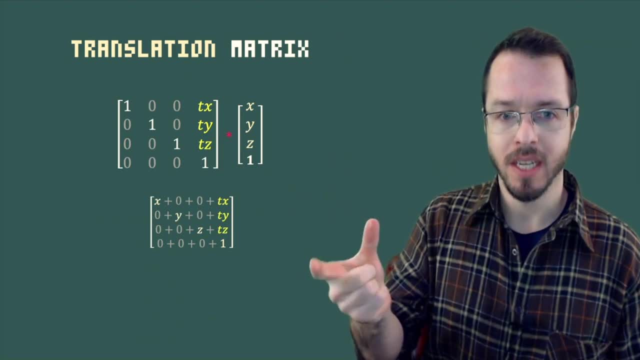 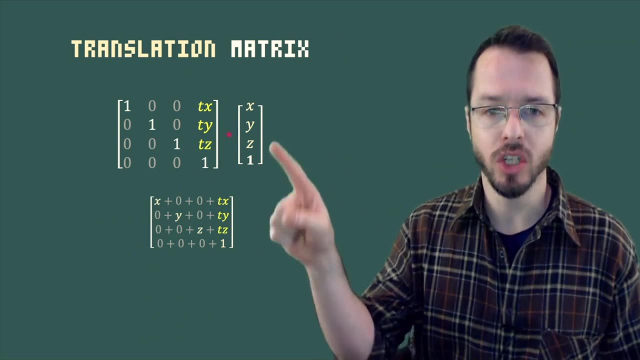 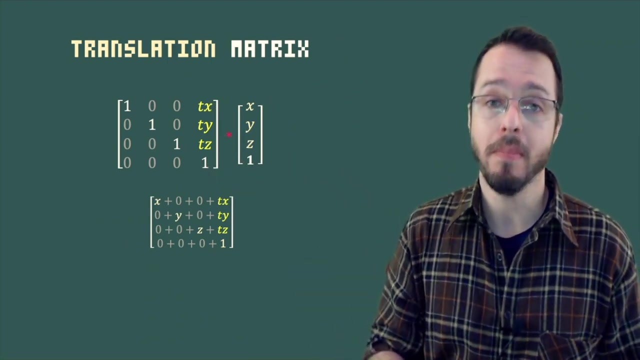 this is x plus the little tx of set. So the only way we could achieve this result right here by adding something right, Adding this tx factor to our original x, is by having this extra column here at the end, And this is one of the reasons, mathematically, why we have to have 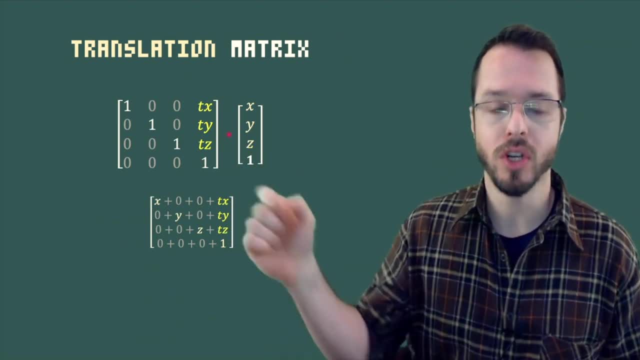 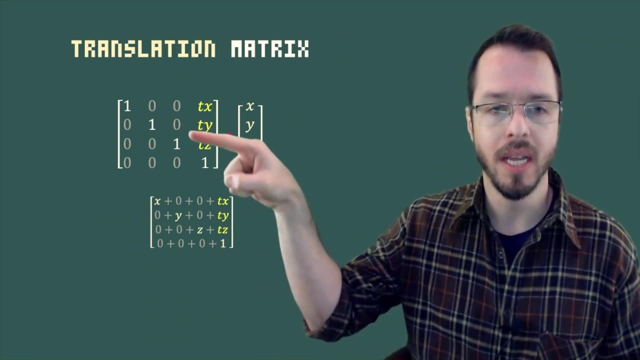 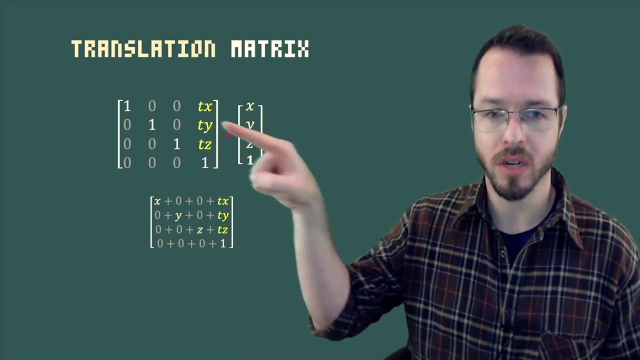 this extra component, why we have to add this extra little column to our original matrix. okay, And if you see, here it's going to kind of follow the same idea, right? So since we have 1,, 1,, 1 in the diagonal, the second row is going to be 0 times x plus 1 times y. Do you see how? now? 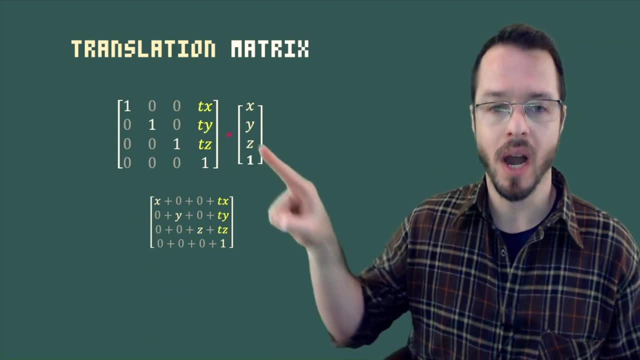 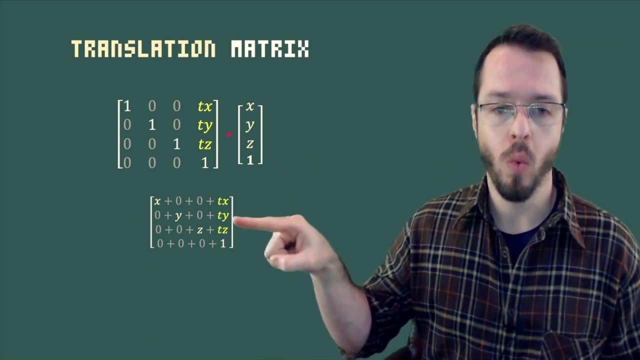 we are considering the y Plus 0 times z plus ty times 1.. So this is this result right here: 0 plus y plus 0 plus ty. So this is effectively y plus ty. So I add something to my ty, Do you see? 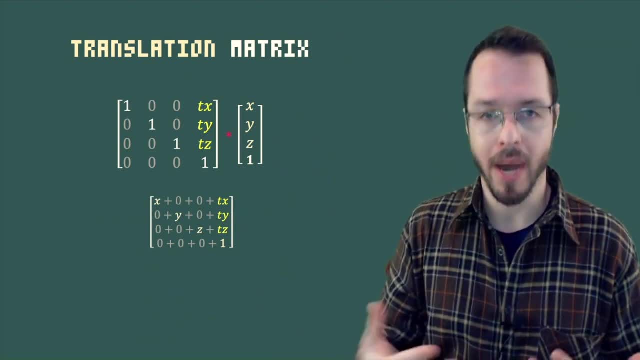 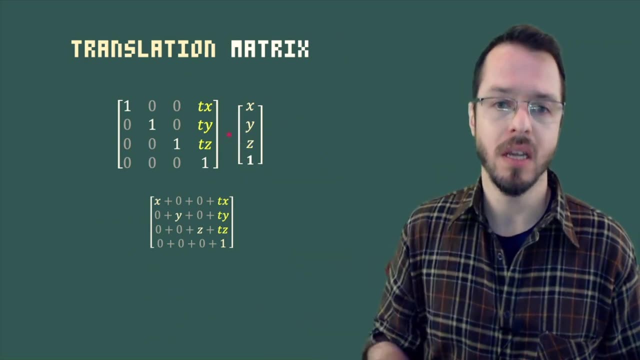 where we're getting. This is, mathematically, why we had to go by the idea of matrix multiplication. The only way that this would work right, That we can add these values, is because we have to add this extra little component. So we add something to the last tx, ty and tz. So if you kind of 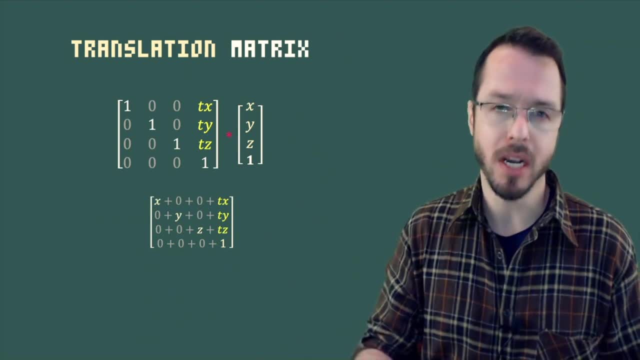 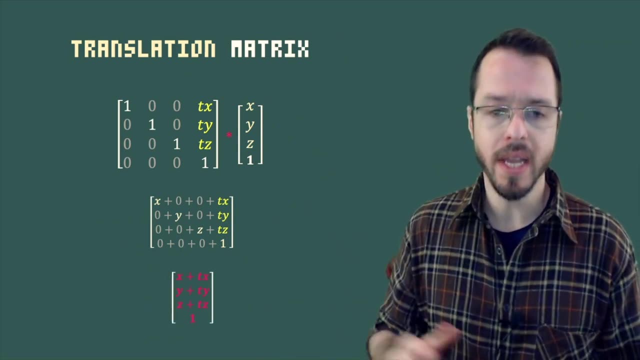 open all these things and I'm just keeping the 1 neutral here because we need to keep that neutral at the end. If we just open this thing, the result of this multiplication, if we open everything and multiply, we get at the end the original x plus how much I want to translate in x- the original y. 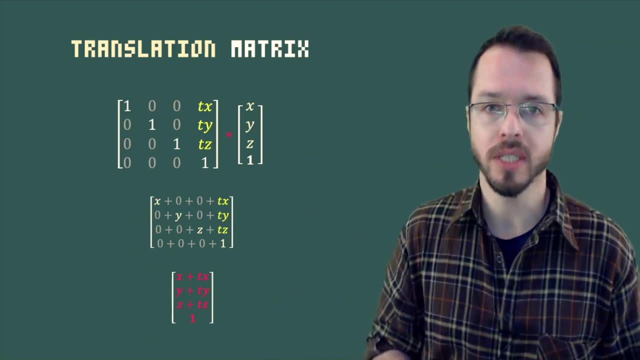 plus how much I want to translate in y and the original z, plus how much I want to translate in z. That thing right. And then of course the 1, we keep that 1 extra, because this is the thing. 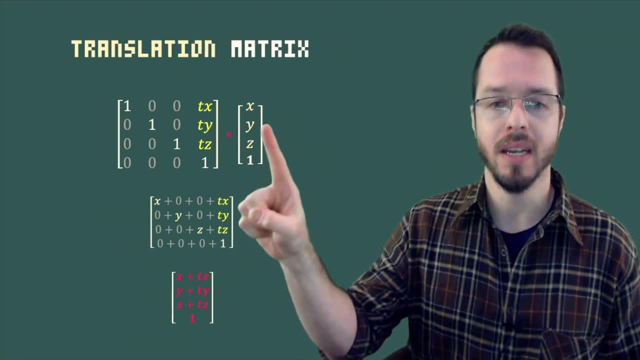 right, Since now we're multiplying a 4 by 4 matrix by a 4 by 1 matrix, we are going to have a little value here. So we're going to have a little value here. So we're going to have a little. 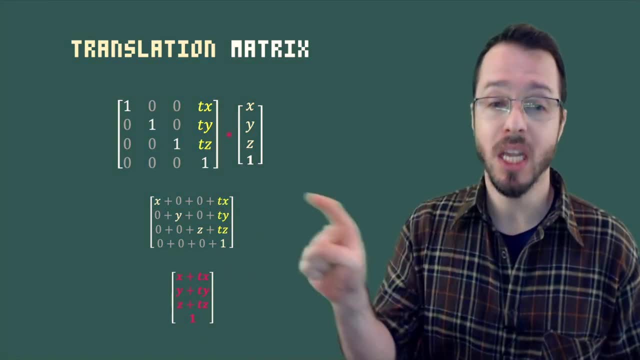 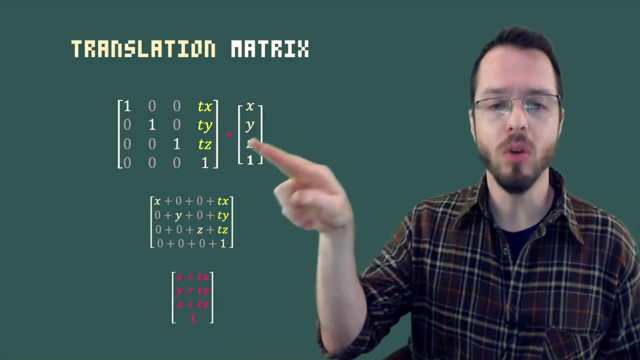 vector 4 with 4 components: x, y, z- and you will see people call this thing the w. So x, y, z and this extra 1 right here, The output right. The result of this multiplication is going to be: 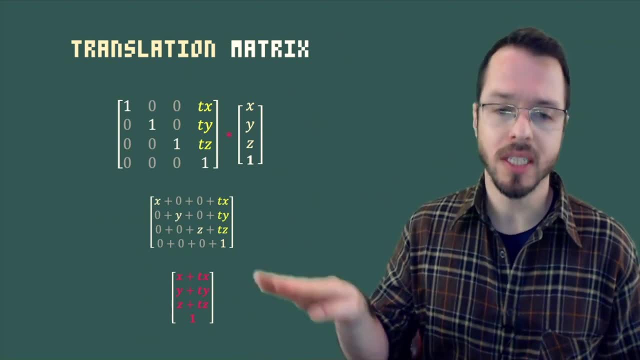 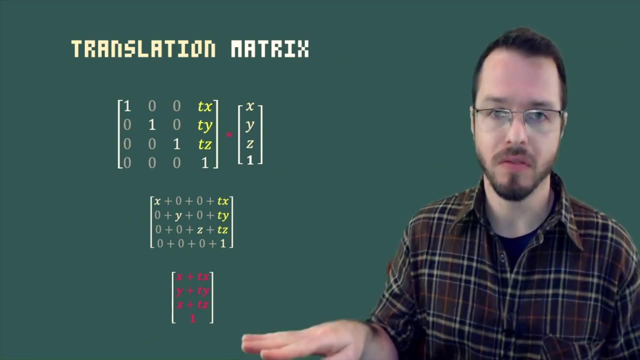 a vec 4.. It's going to be a vector of 4 components And you're going to see that people call this thing as part of these ideas of homogeneous coordinates. right, And homogeneous coordinates, this vector 4, they are going to be all over whenever we are going to start working with. 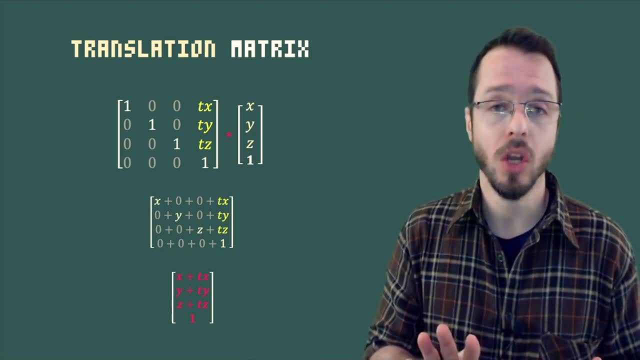 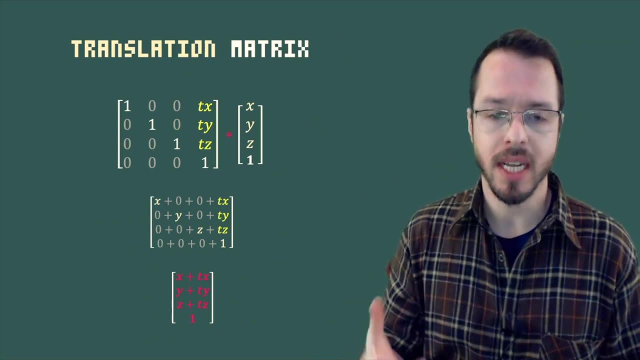 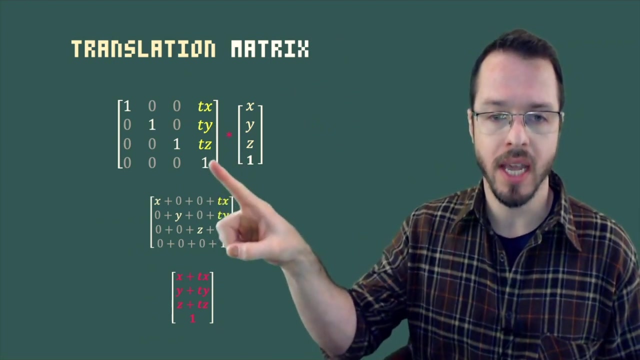 matrices projection in 3D computer graphics. But look this thing right. here is the mathematical reason why we need a 4 by 4 matrix. right, Because if we understand that the only way that we can actually get and add something at the end is by adding this extra column with 1 here at the end. 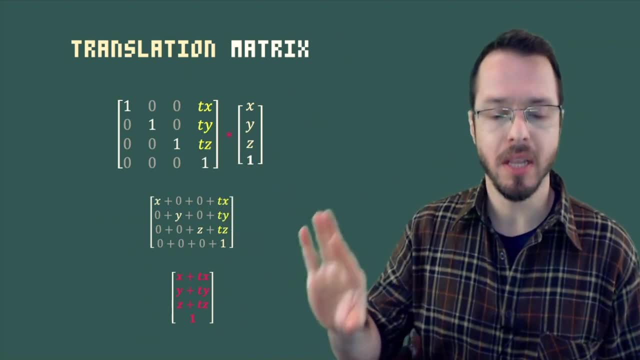 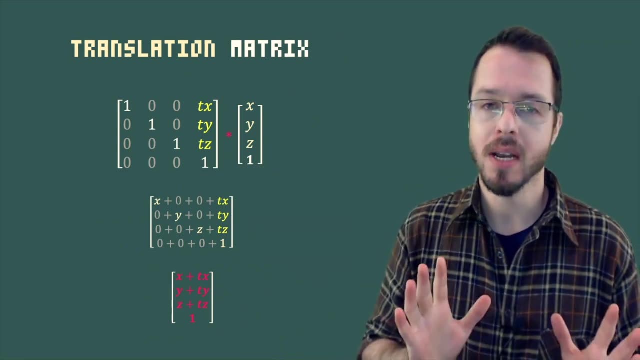 with these real factors t x, t y and t z. This is mathematically by expanding in matrix multiplication. This is mathematically why we need to have a matrix 4 by 4.. But that is not. 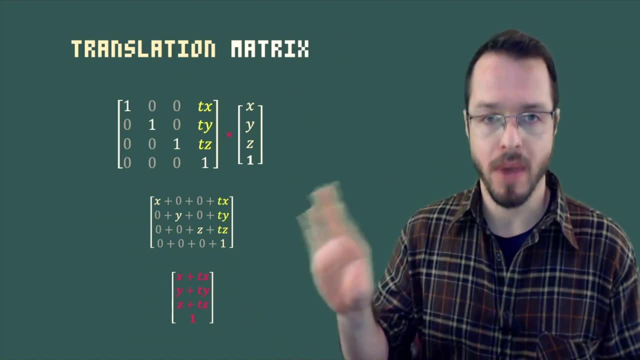 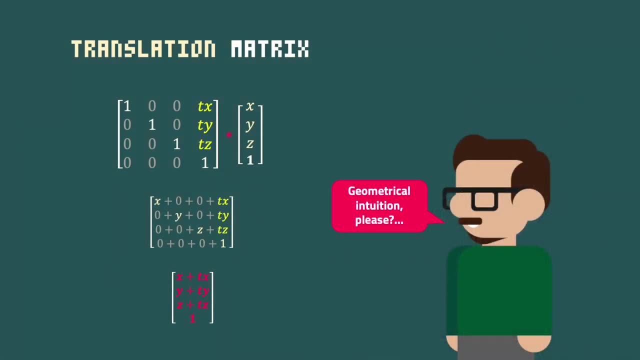 the only thing I want to explain here. I want to, besides having the mathematical explanation of opening the matrix multiplication, I want to also create some sort of intuition, right, Some geometrical explanation of why we have this 4 by 4 matrix as well. right, I want to explain that using this kind. 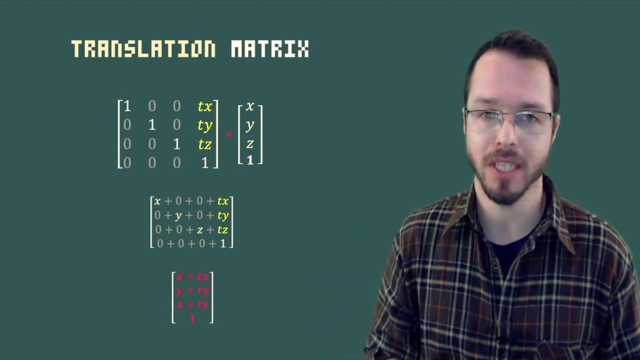 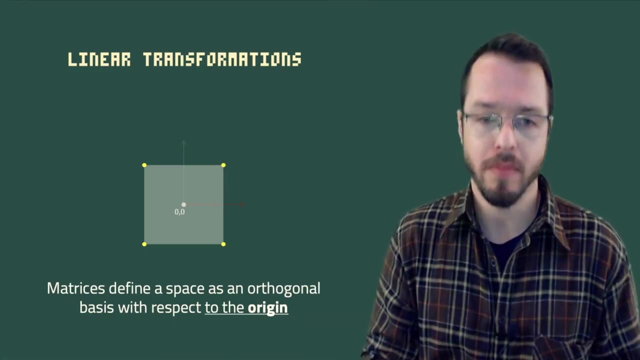 of visual approach. what is the reason why we have this 4 by 4 matrix And, look, this is going to be super cool. So let's go back a little bit and let's talk about these ideas of linear transformation. Remember when I said these things about scaling? 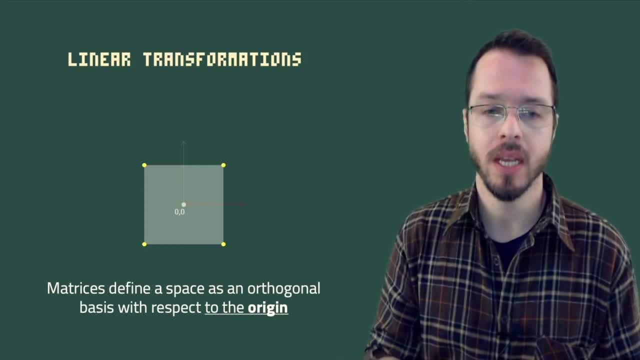 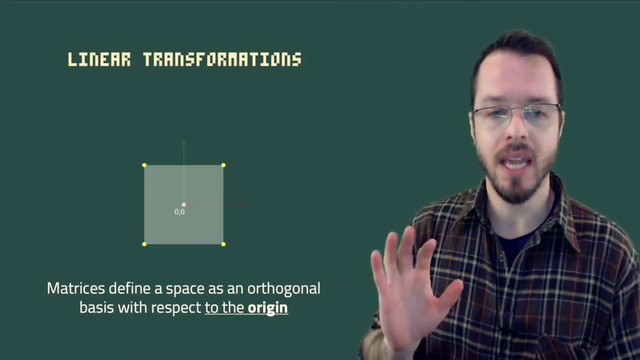 vectors, rotating vectors and translating vectors. Look, we are using these ideas of linear transformations. right, And remember that, from mathematics, linear transformations, they are that thing that we can apply to vectors. we can apply to these linear values and we are. 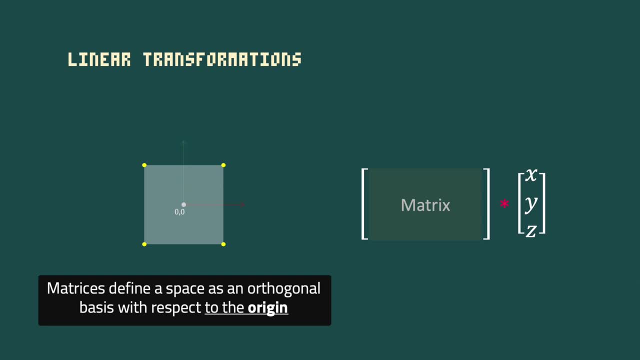 effectively using matrices to represent these linear transformations. Remember that we have these matrices and then these matrices. they are the ones responsible for applying scaling, rotation, translation and etc. right, These linear transformations. So look at what it says there. It says matrices define a space as an orthogonal basis with respect to the origin. 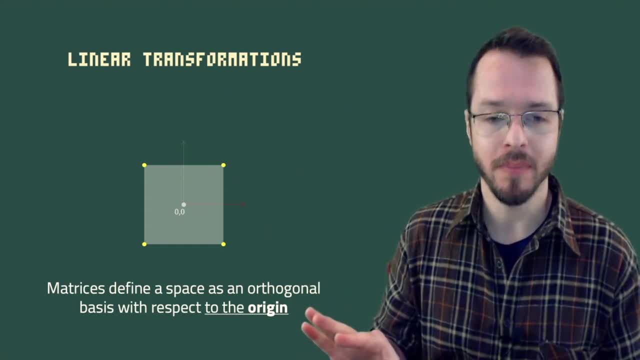 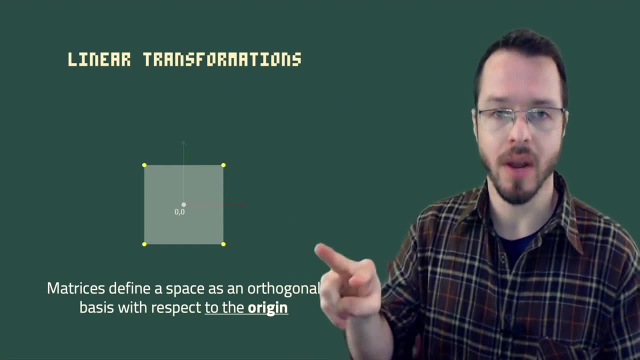 And that is a mouthful sentence, but basically what this means is matrices. they apply the transformations, but everything is with respect to the origin. We cannot change the origin, our center right. So look at this: Do you agree that rotation, whenever we rotate things? 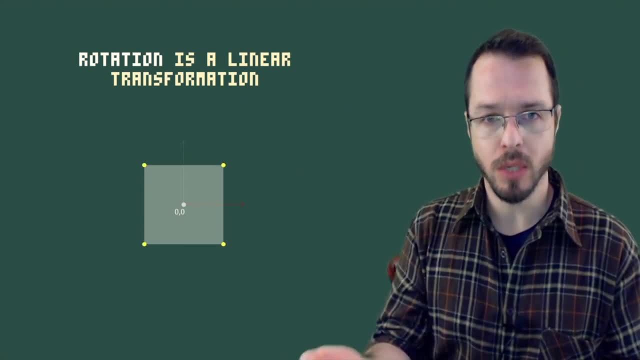 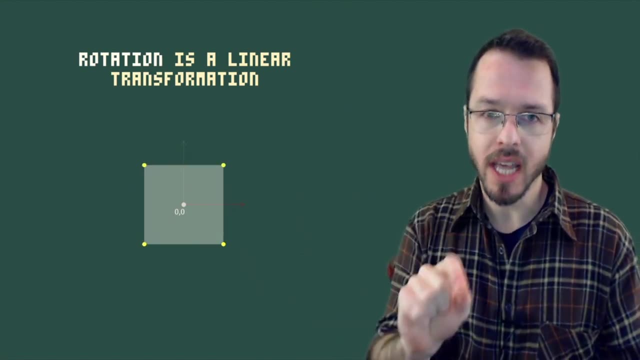 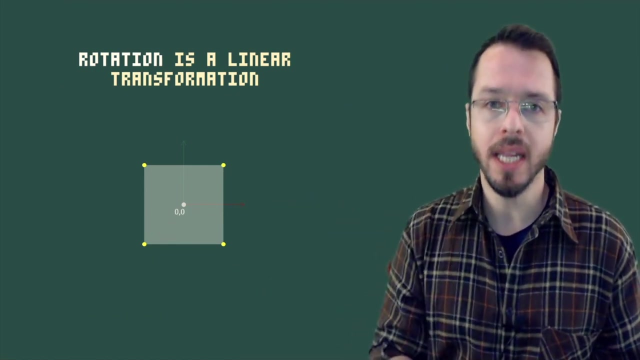 right, This thing, right here: When we rotate those points and we apply the transformation, do you agree that the origin doesn't change, right? So if I go and I rotate things, my origin stays there right In the center. Of course, zero times zero has to be zero. So this is, of course, a pure linear 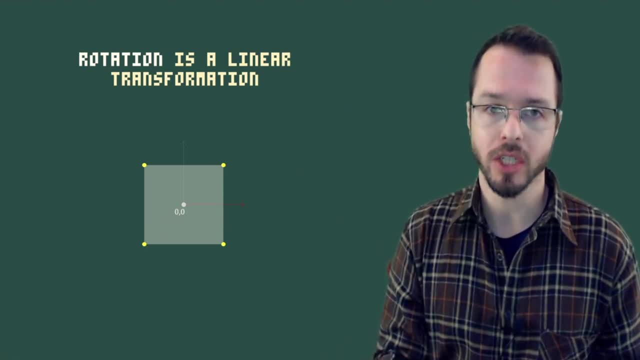 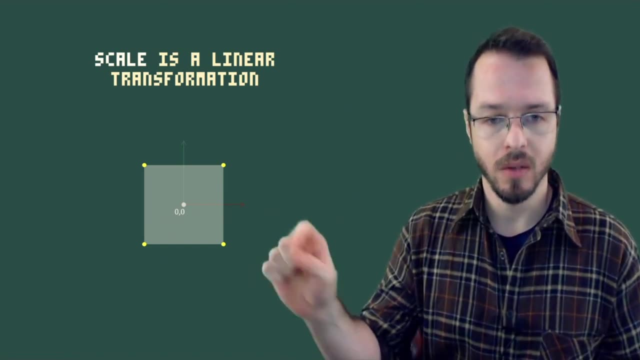 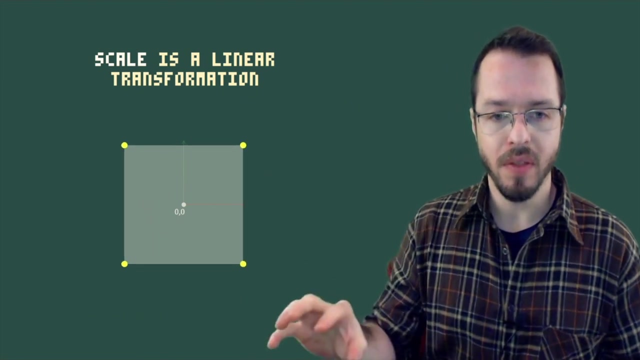 transformation. So rotation is indeed a linear transformation. What about scaling? Well, scaling, of course it is as well linear transformation, because again, we start with lines, we end up with lines and we, We also have that center right, We don't change anything. Everything is this orthogonal basis. 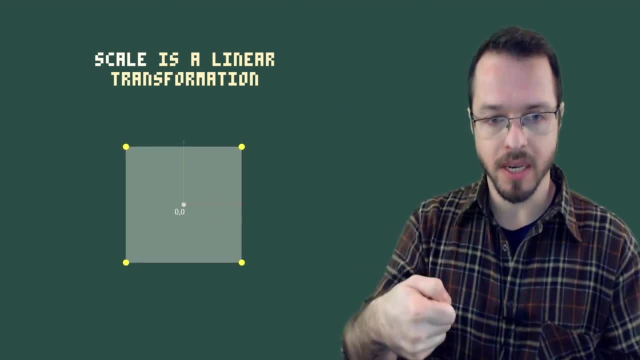 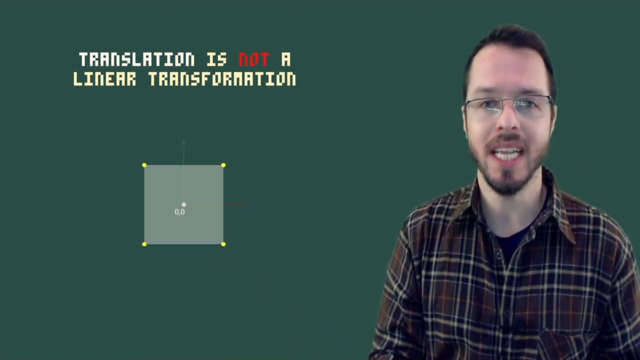 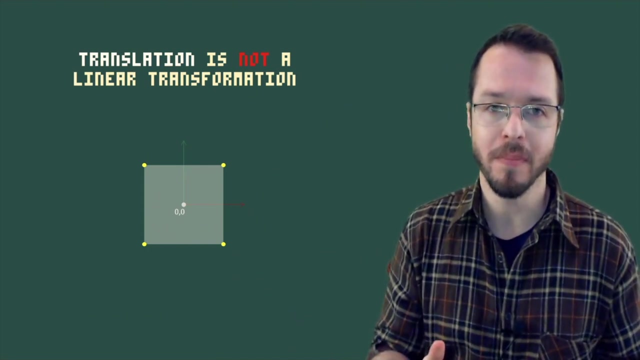 with the center unchanged. So I go and I scale things up and down, but the origin is still always there. The problem is translation, right? So translation it is not a linear transformation, right? And look, I have been calling translation linear transformation before in the course. 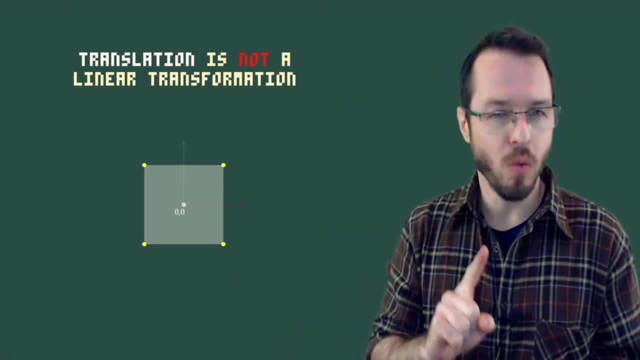 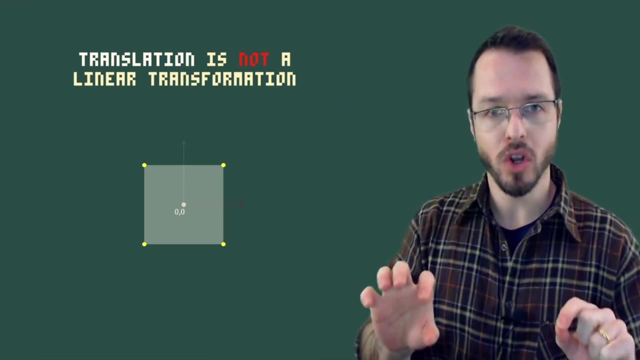 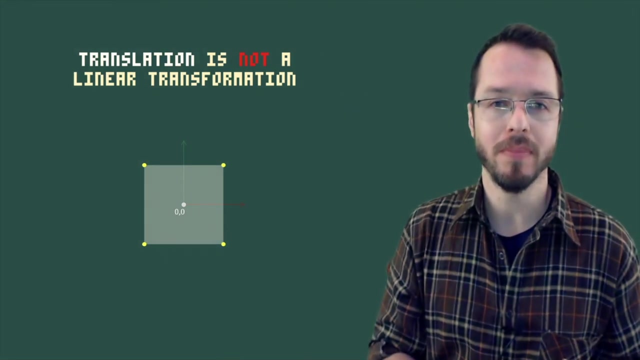 but I was basically lying to you. right, Translation it is a weird one. It is not linear transformation because the translation, if you translate those vectors around, we are gonna change the origin. right, The origin keeps the same, but the object changes the position. So that is a little problem and 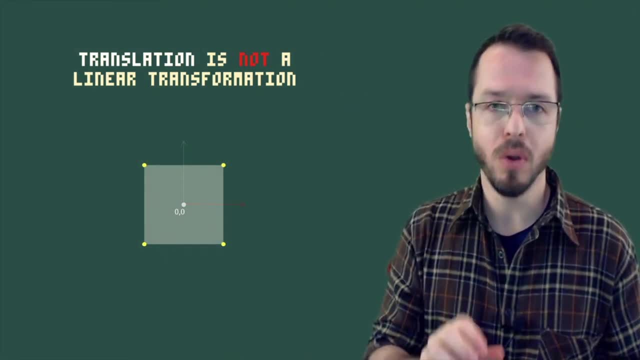 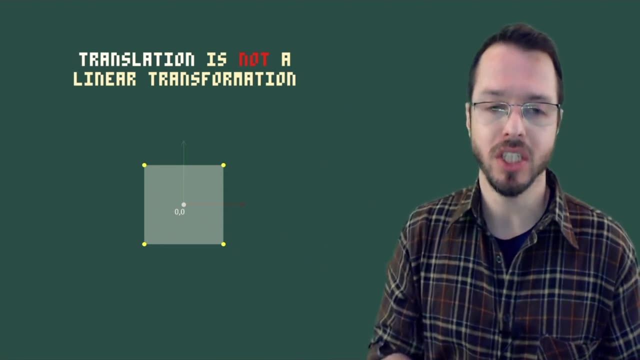 this is one of the reasons why we cannot have a simple tree by tree matrix to represent translation. This is one of the explanations. right, Geometrically, this is one of the explanation why we need a four by four matrix. But I wanna go even further, right? I wanna explain why. 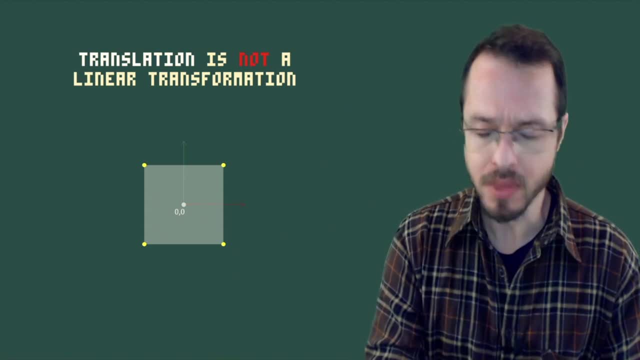 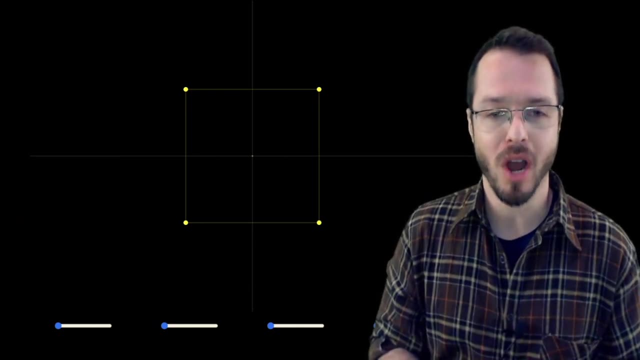 do we have these ideas, And for that I want to give an example. I'm gonna read you an example example. I need to talk to you about something else, So I created here a little applet, right, A simple applet using the browser. So this is the thing: If we have this little set of vertices, 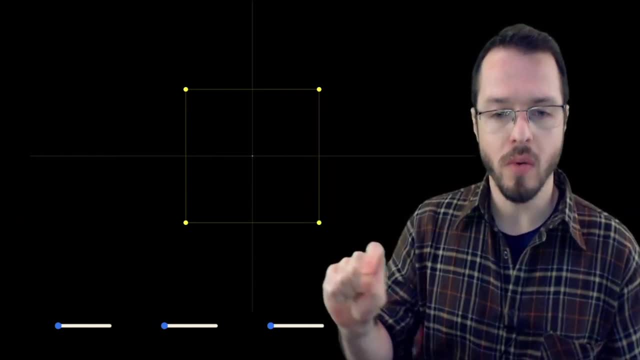 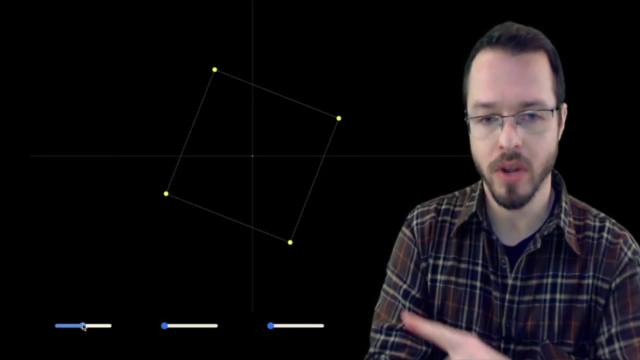 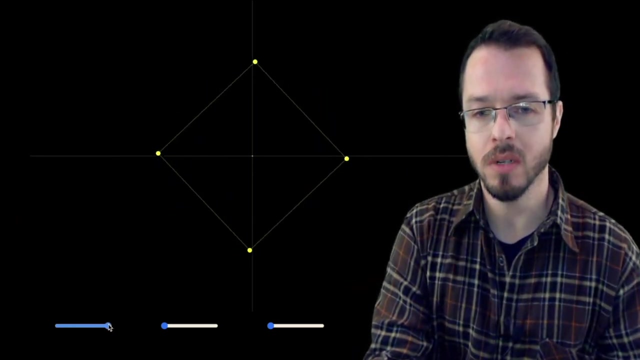 right, I have four vertices: one, two, three, four. They are all in this X and Y positions. And then look, if I come here and if I perform a rotation, we agree that my origin stays the same. so everything is changing. I rotate my things by a certain angle. right, I can also think about 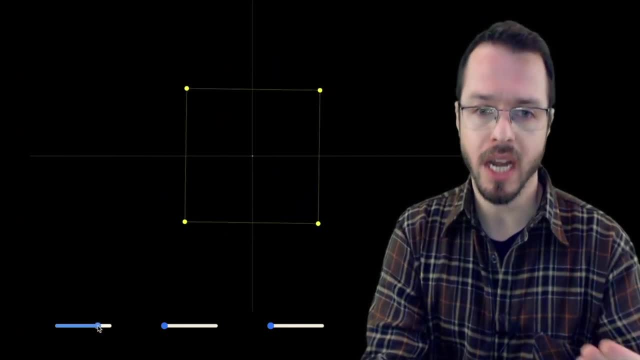 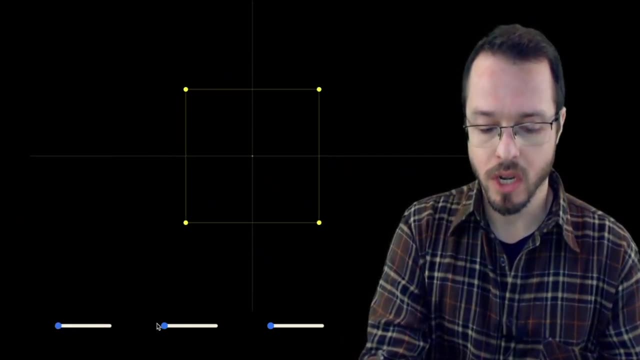 this, right, I'm performing a matrix multiplication so I rotate by an angle, but my origin stays the same. That is rotation, right. If I want to perform scaling- kind of the same thing, right, I can scale things up and down, My origin stays the same. That is what we just 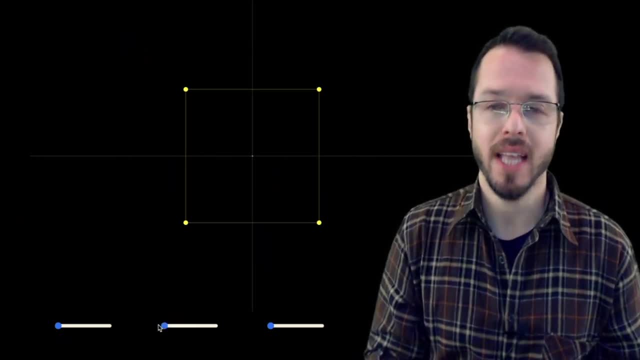 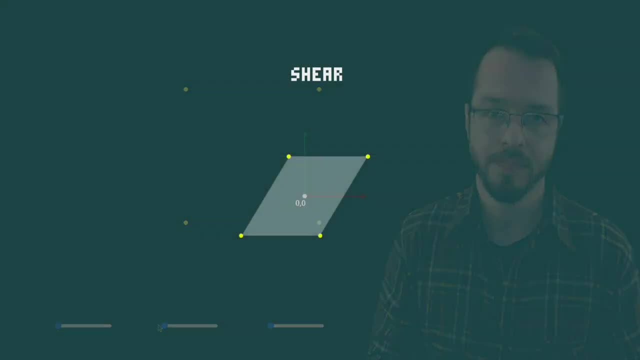 discussed. There is another transformation that it is not very well, It's not very popular, but we need to discuss, which is called shear. So shear is a transformation that we can apply, which is a pure linear transformation, because look at what happens whenever we have to. 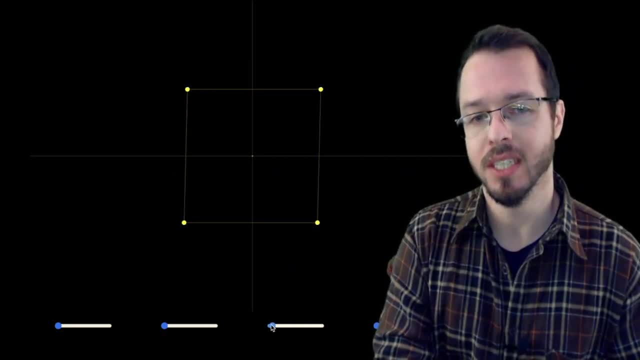 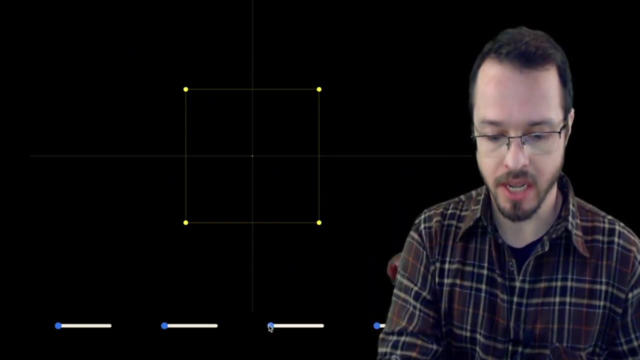 shear things in our objects. This is the result of shearing. It's almost like I go and I skew things right. I go and I distort them. So this is me shearing in X: I go there and I shear things around. So do you see? the origin stays the same, right? This is a pure linear transformation. 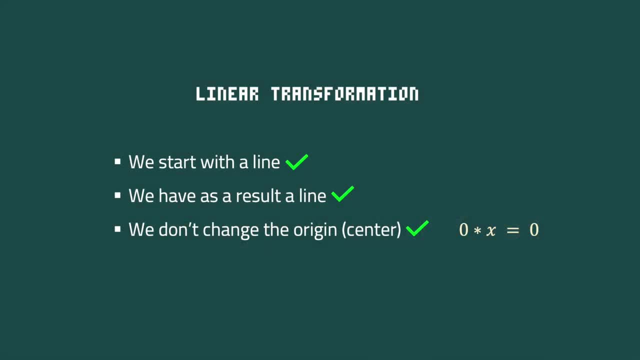 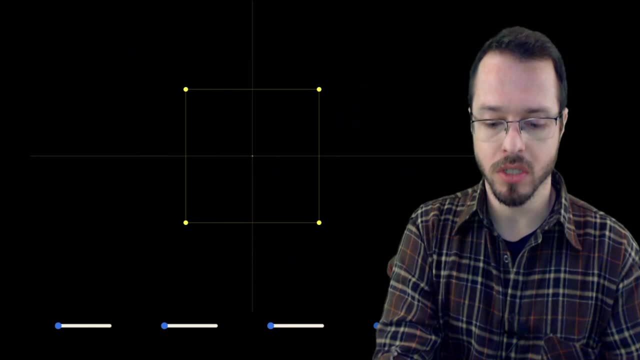 starts with lines, we end up with lines, but my origin is always at the center, unchanged. So if I go here and I skew in X, this is what I get. I can also come and skew in Z, right? So it's just a. 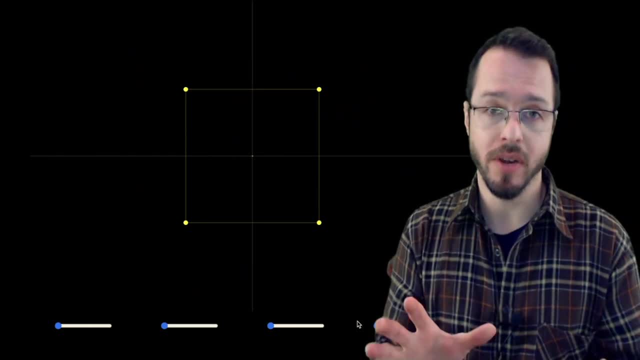 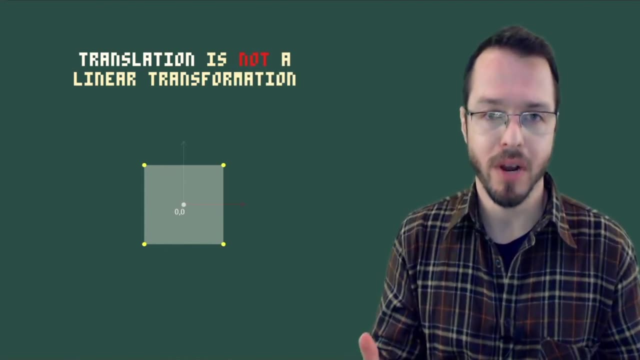 little different skew, but that is the whole point. This is shearing, right. This is a shearing transformation. Gustavo, why are we talking about shearing now? right, If we were talking about translations before- and translation was the little odd one out- why did we open a little? 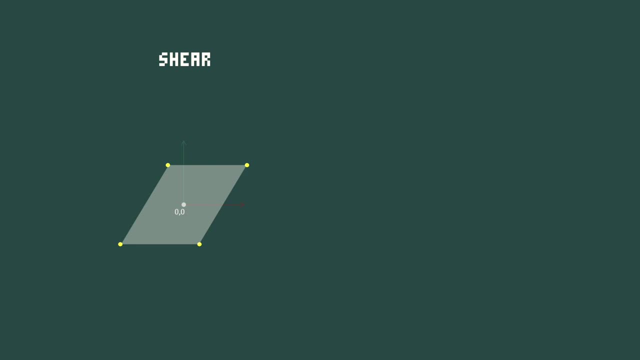 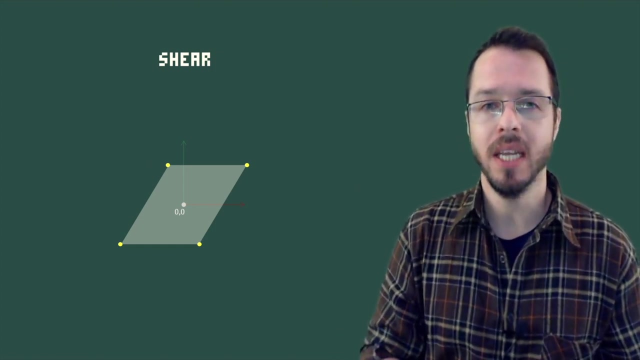 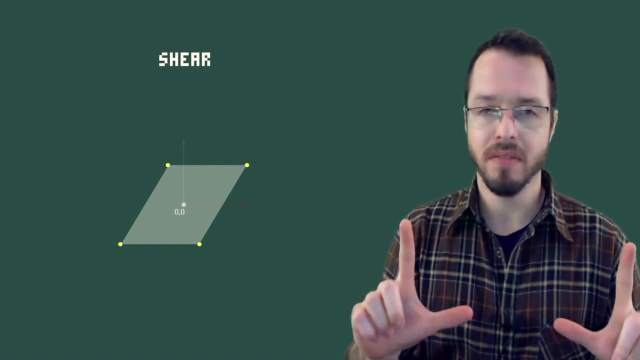 parenthesis. and why are we speaking about shearing transformation? Because there is this very smart trick that we can use, that we can represent a translation by means of shearing. And I'm going to propose a quick mental activity. Think about this. Think that you have a little. 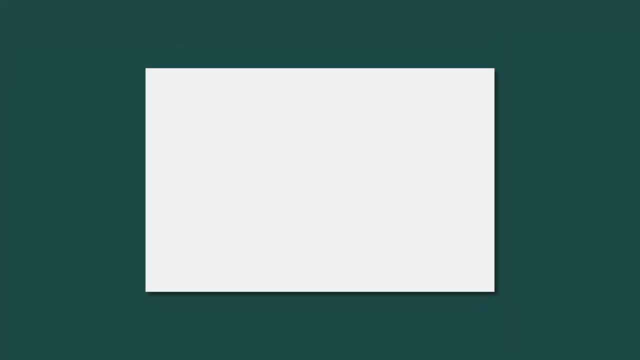 piece of paper with you, right, This 2D piece of paper, And I want you to think that we add four points to this piece of paper: four vectors right, Four little vertices, And these four vertices, they have X and Y positions, And do you agree that we cannot translate this thing? 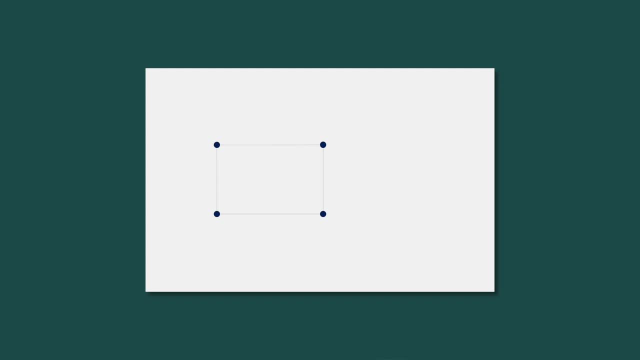 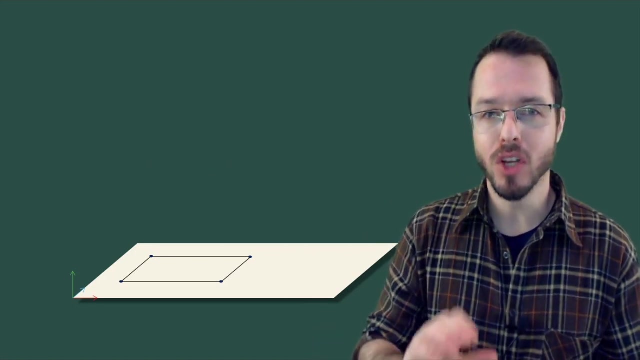 using a linear transformation right In this 2D plane. A translation is not a linear transformation, So I cannot translate this little rectangle around, But what we can do is- and look how cool this is- We're going to raise this problem one dimension So, instead of 2D. 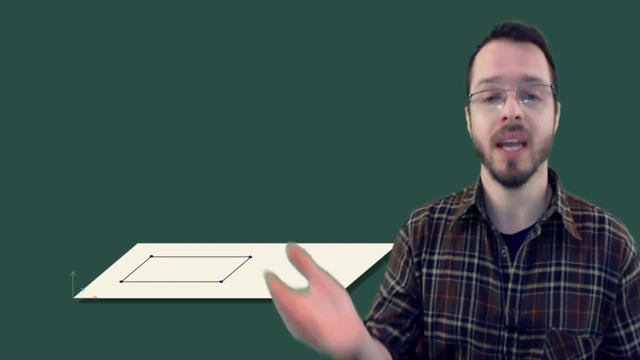 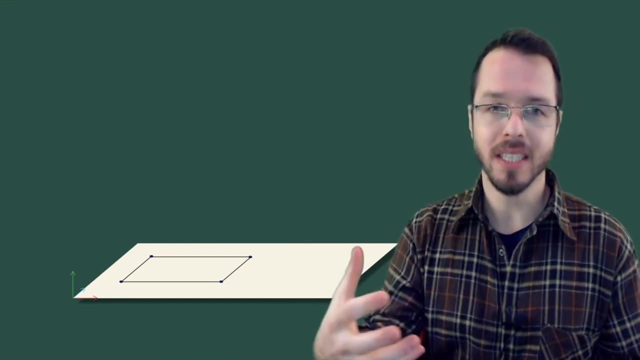 we're going to go to the next dimension, which is 3D, And I want you to think about again that piece of paper, And then we end up with this 3D aspect right here. So we raise that problem one dimension up right. So now we are in 3D And whenever we are in 3D, I want you to 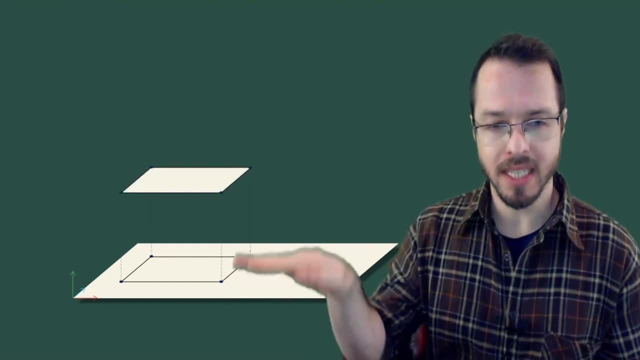 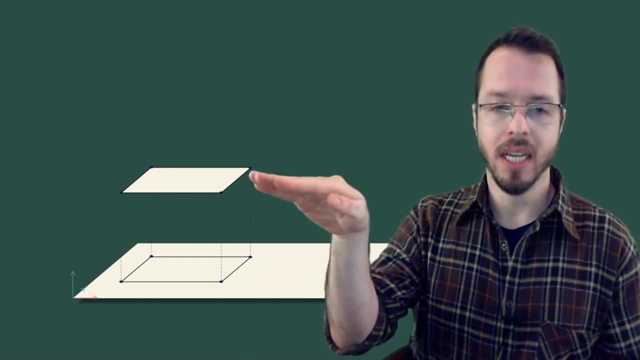 think about offsetting this thing. right, I want you to think about offsetting this little rectangle, the vertices up. So do you agree that now that we are in 3D and we have this little offset here, do we agree that this and we end up with this area right here, right, We have this kind of 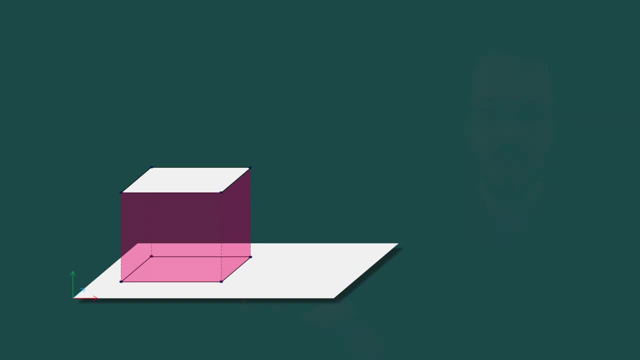 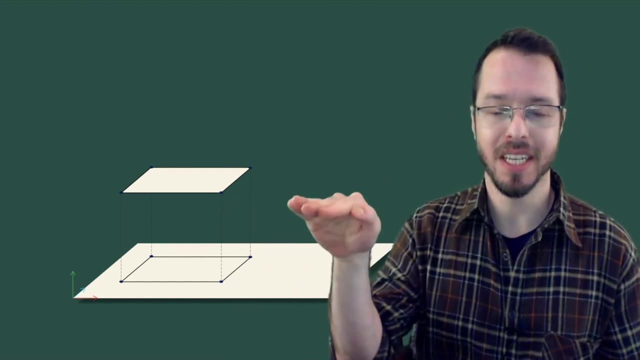 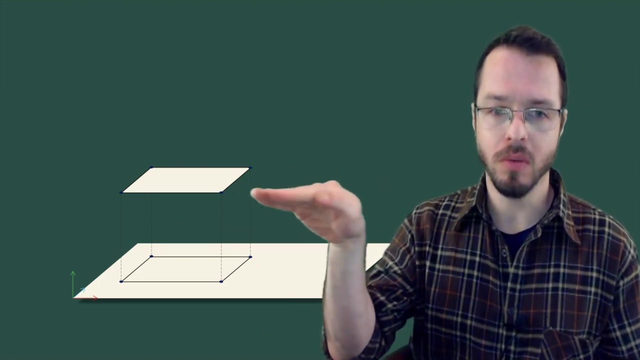 cube rectangular surface, Solid right here. Now that we are in 3D, I want us to think about shearing this little shape here to the right. So if we apply a shearing in this three-dimensional space, right I go and I apply. 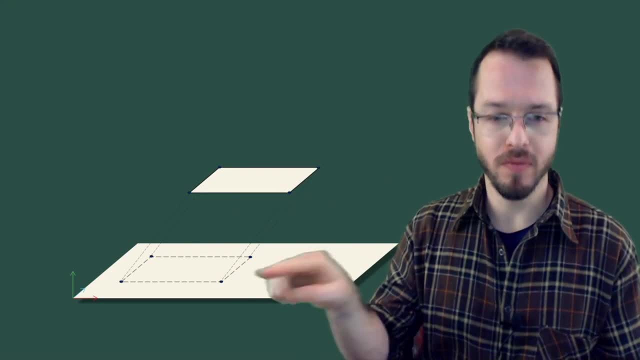 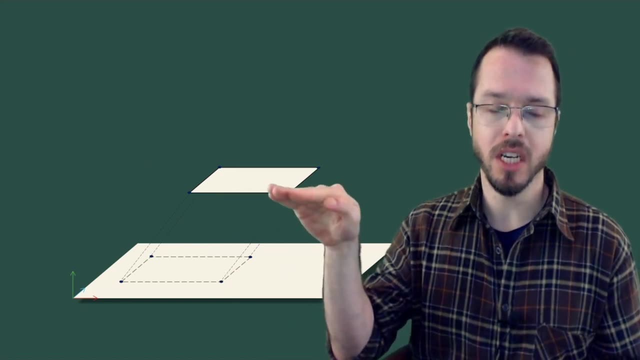 this little shearing to the right- I end up with this right. So think about your origin- is still our base right, So we still have that thing there. That was our origin. Now, we performed a little shearing in 3D. 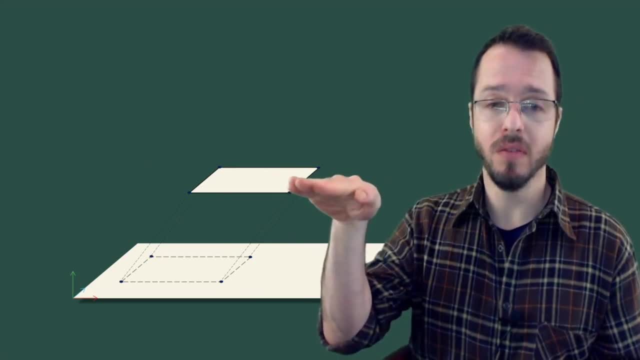 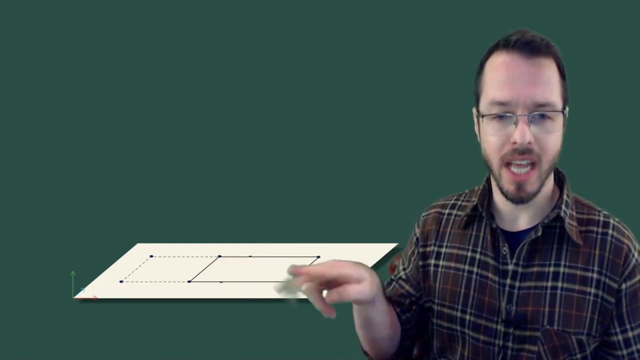 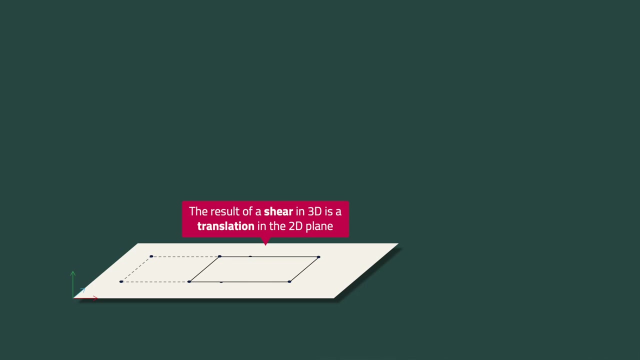 And now that we performed a shearing in 3D, if we go back to 2D, do you agree that, if I flatten things out, this is actually a translation of that original thing? And look, I know that this changing of dimension is not something that we see every day, but I wanted to think about this. 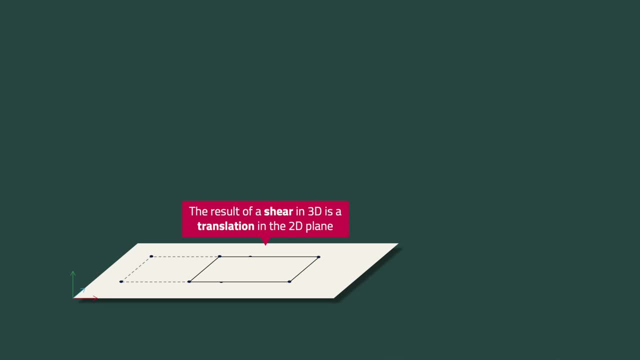 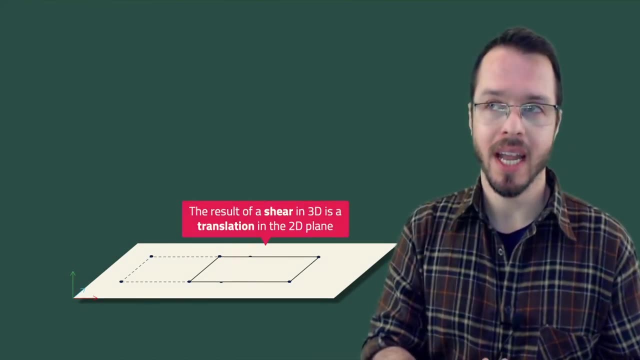 right. The result of a shear in 3D is basically a translation in our 2D space. So we start our 2D And for us to perform a translation in 2D, we're going to raise that problem. one dimension. 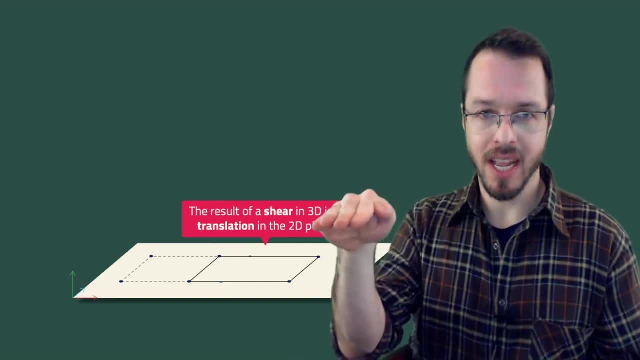 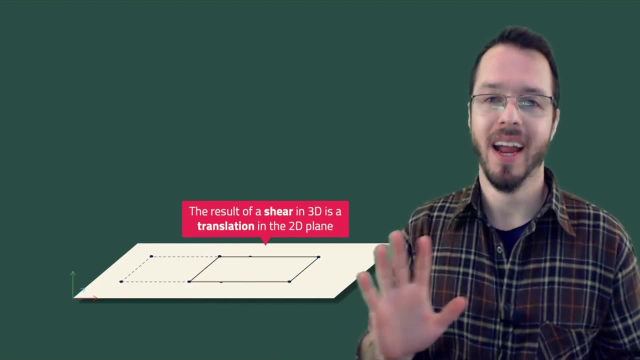 So we're going to go to 3D, We're going to perform a shearing And then if we go back to 2D, that is indeed a translation right. We basically translated something to the right And look the even cooler. 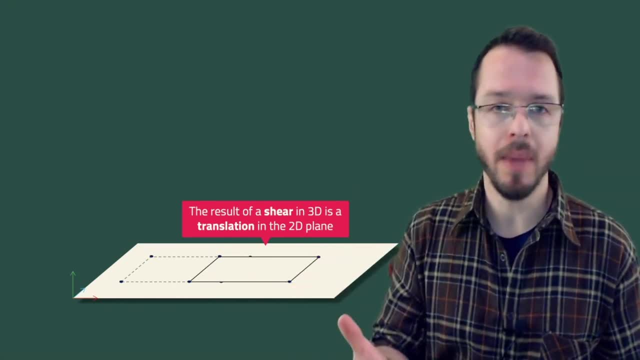 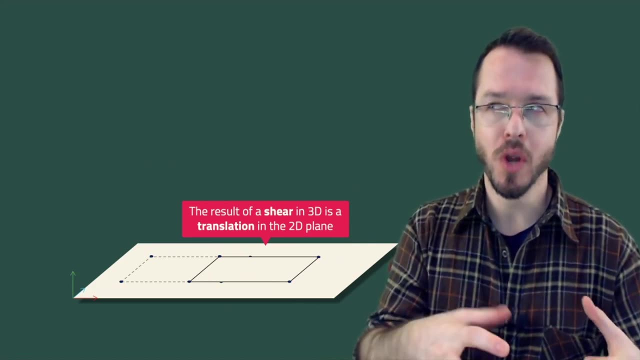 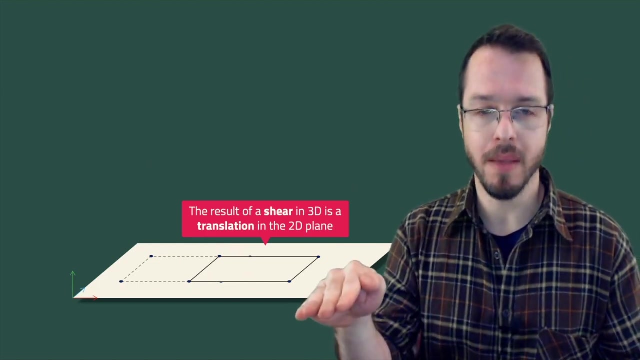 thing is. this thing holds true for any dimension. So if we have a 3D problem, right, If we have 3D points and 3D vectors, we're going to Raise this thing to the fourth dimension And then we're going to perform a shear in the fourth. 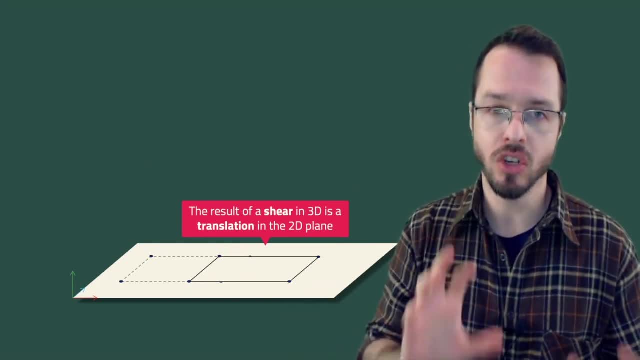 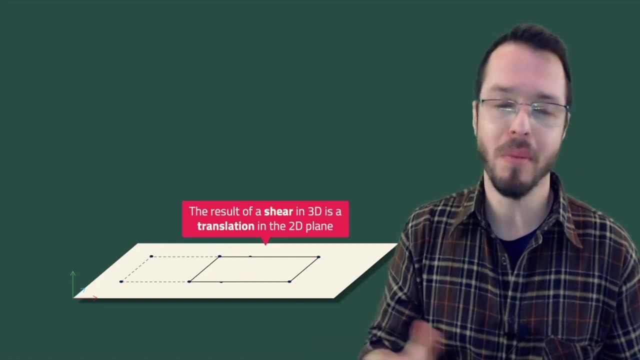 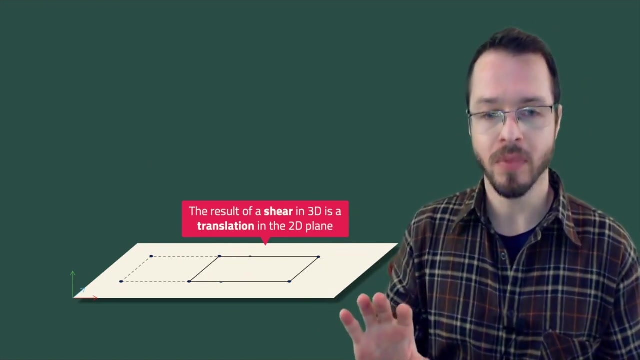 dimension And then when we come back, we have a translation in 3D. And if this is not the coolest thing you've heard this week, I don't know. you probably have a lot cooler week than I do, But I think this is super cool because this is basically the explanation of why we have to go to 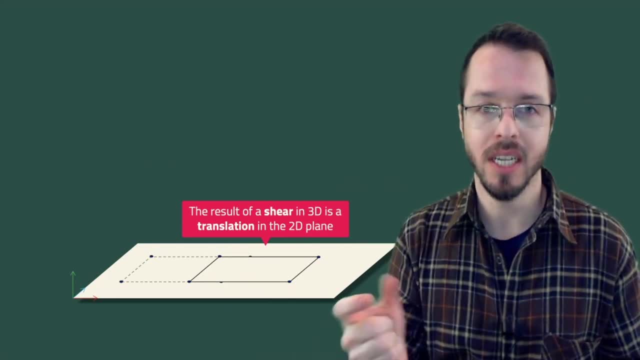 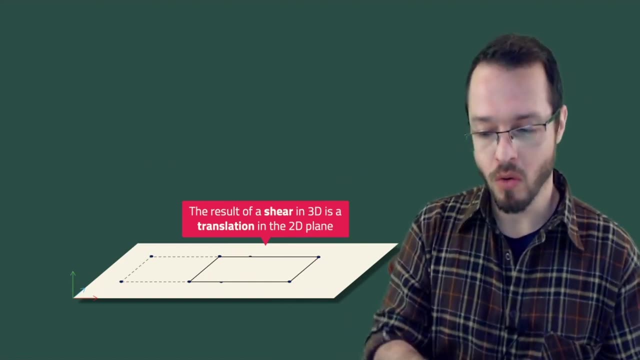 this fourth dimension to perform a translation in our 3D space. So if we go back to 2D, we're going to 3D world right, All those 3D vertices. we have to have this 4x4 matrix because we are raising the 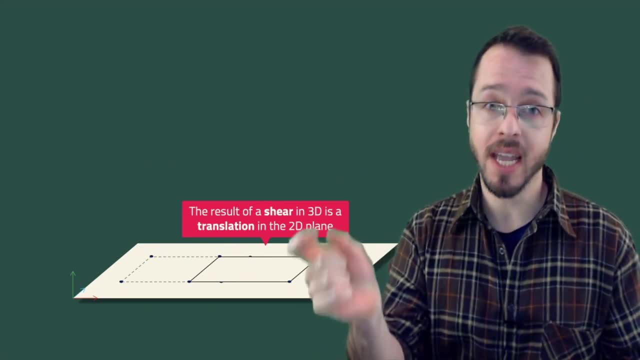 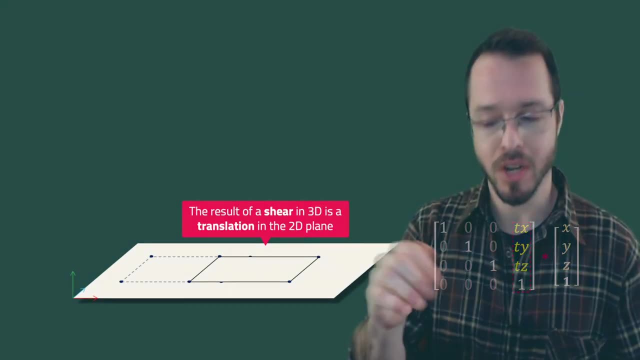 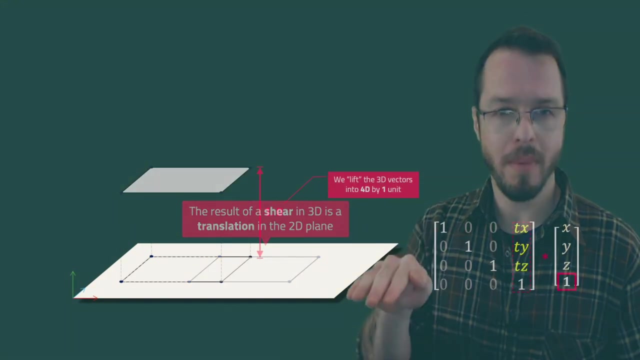 problem: from 3D to 4D, performing a shearing at the end, That transformation that we apply at the last column is actually a shearing right. We are shearing that thing, We are shearing those vectors that we have, And then we are coming back right. So we go, we apply a little offset of one, Do you? 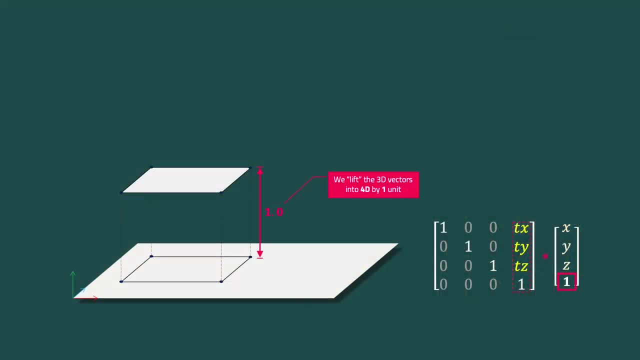 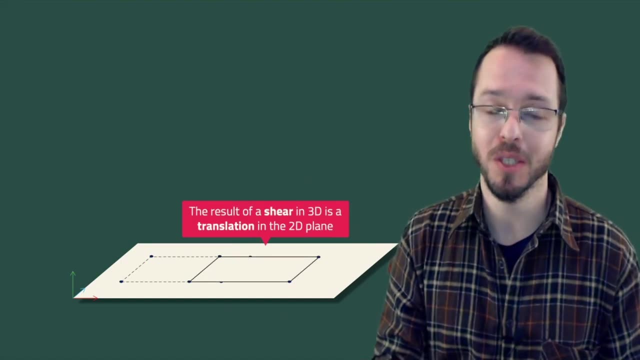 remember how we have that one at the end. So we go, we raise by one, we perform a shearing and then we go back to 3D And that is basically us translating things using- well, we are using a matrix, but we are actually performing a shearing in four dimensions Because, as we saw before,